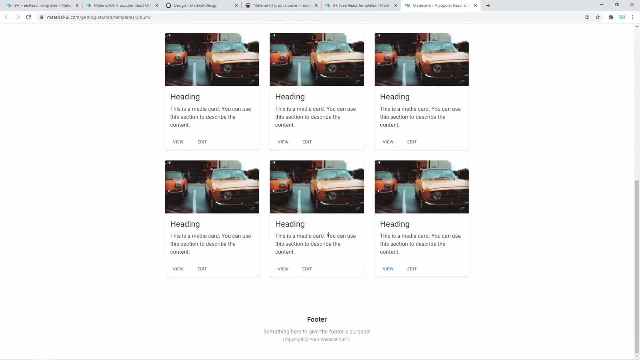 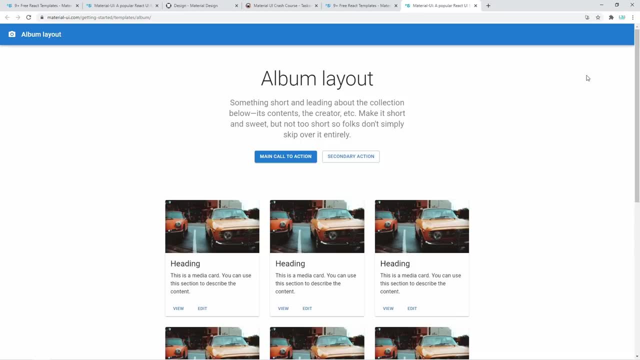 buttons and how to create these nice looking cards, as well as the footer. This one simple project is going to teach you not only what Material UI is, but also how you can immediately start using it on your own projects. This video is special because it acts as a practical guide to get you 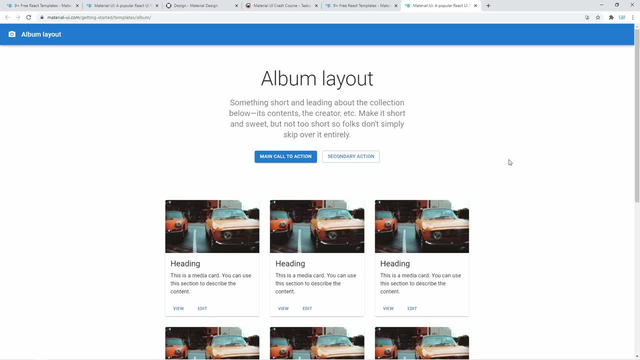 up and going with Material UI. You're not only going to learn things to learn them. you're going to learn them so that you can put them into practice and immediately start using them in your own projects. If you've been subscribed to JavaScript Mastery for quite. 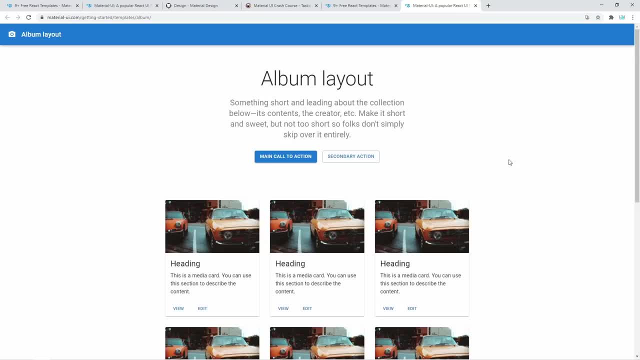 some time now. you know that that is the way that we do it on this channel Project only. If you're still not subscribed, well, now is the time to click that subscribe button so that you can be sure to not miss any of the newest projects. Material UI is built by following: 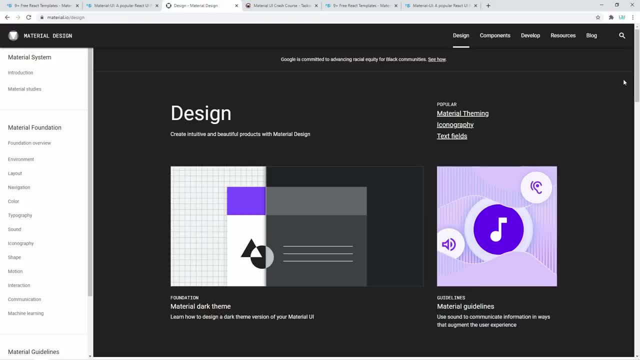 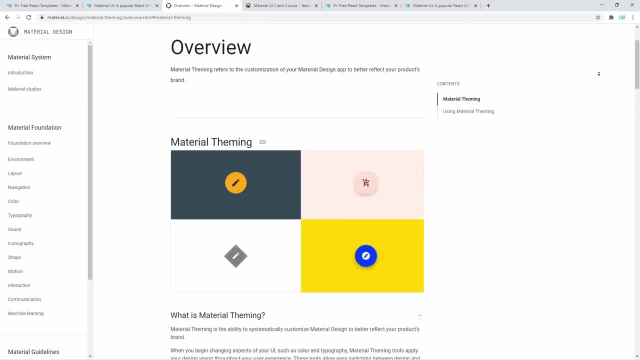 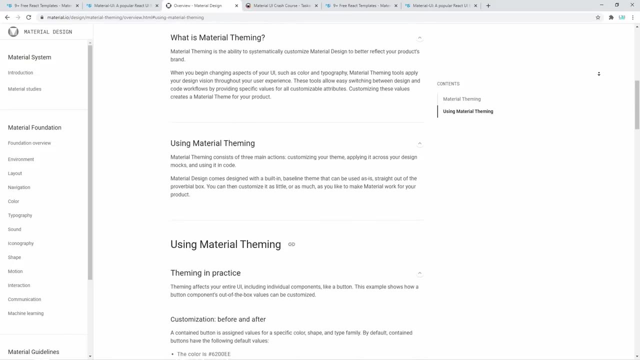 material design guidelines. Material design is a system created by Google to help teams build high quality digital experiences, As you can see on the screen. material design provides guidelines for colors, typography, shape and much more. By following their principles, you can use numerous components that look good and feel good to use. If you'd like me to create 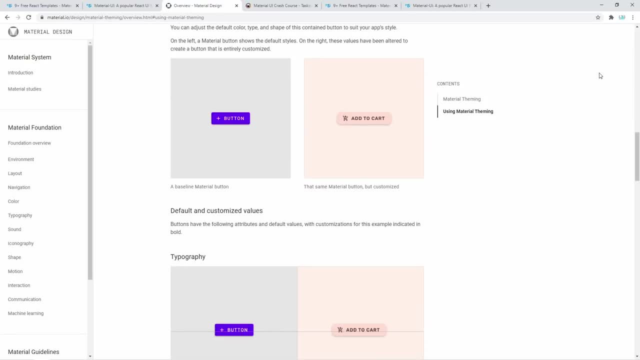 a second part where I go into some more complex Material UI features. make sure to comment and subscribe. If this video reaches 5000 likes, we're recording part 2.. With that said, I only have one more thing I want to let you know, and we'll jump straight into the project. Alongside teaching you. 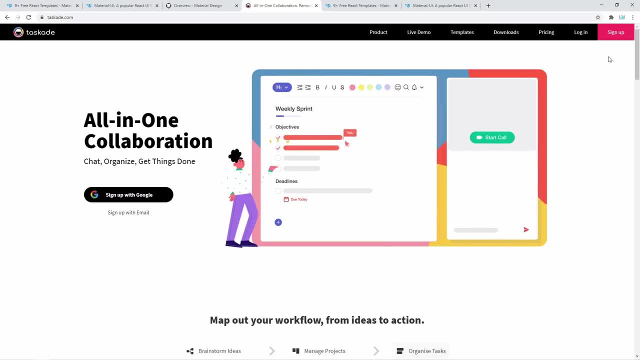 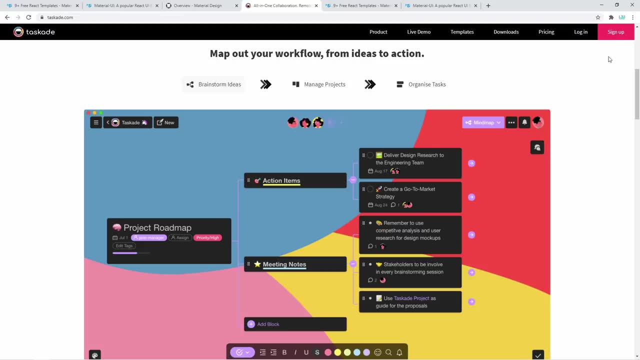 Material UI. in this video, I'm also going to show you how to use Taskade, an all-in-one collaboration tool. I partnered with them and made sure that all of you guys get the pro version. the only thing to get Taskade Pro for free is simply contact Taskade and let them know the JavaScript Mastery. 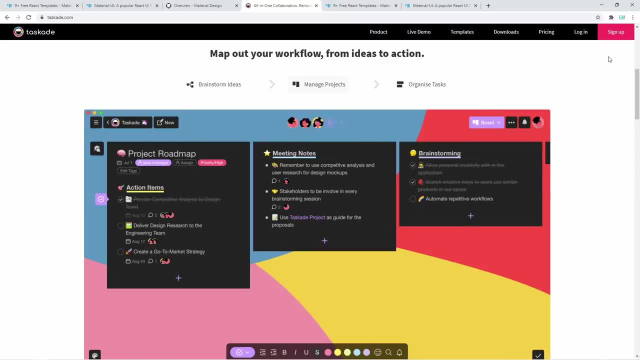 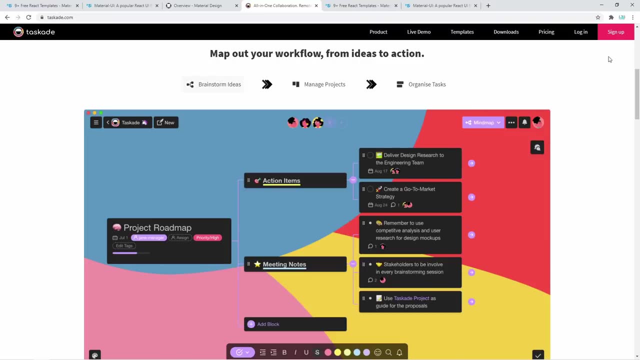 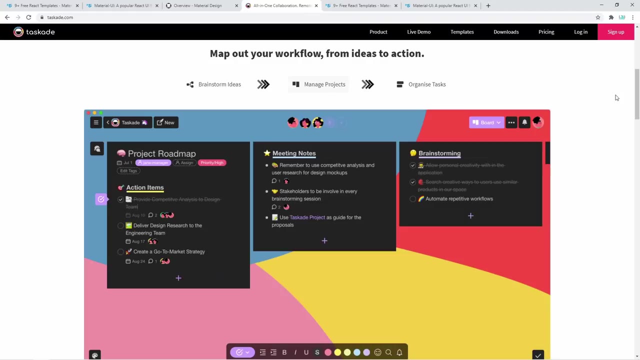 sent you. So what are the main features of Taskade? You can map out your workflow from ideas to action. You can customize the view all the way from a simple task list to any more complex workflow, like a board action or a mind map. It is built for collaboration. 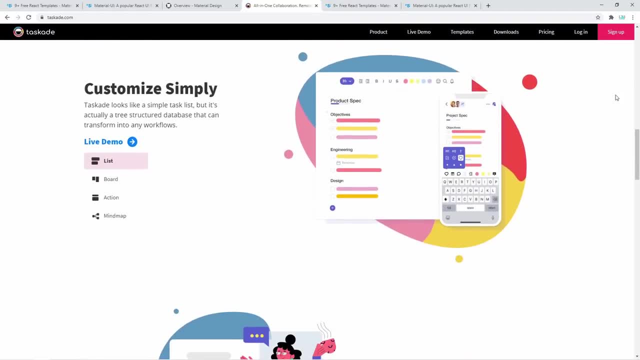 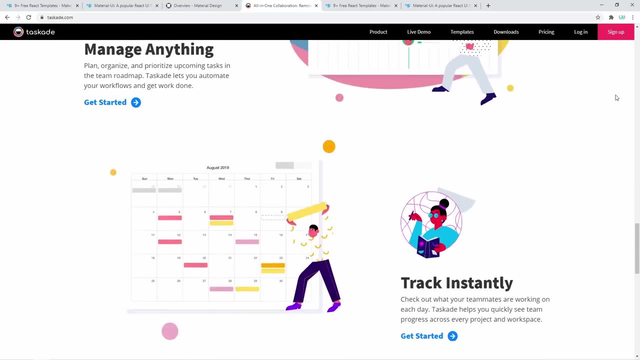 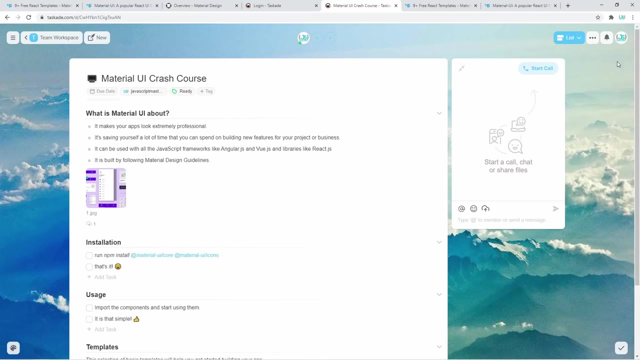 you can see what each teammate is doing in real time. It has amazing calendar views so that you are always up to date with what needs to be done. Taskade is also available on all the major devices and operating systems. Later on in this video, I'm going to show you how to use Taskade while we go. 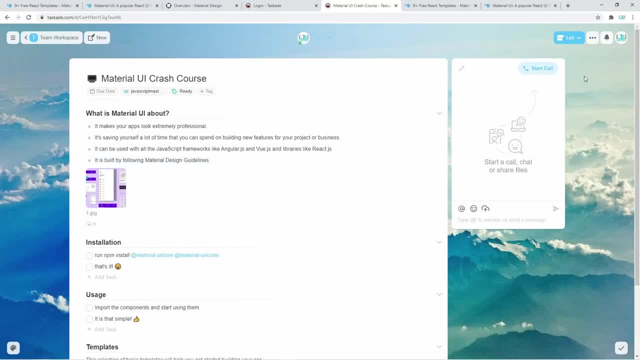 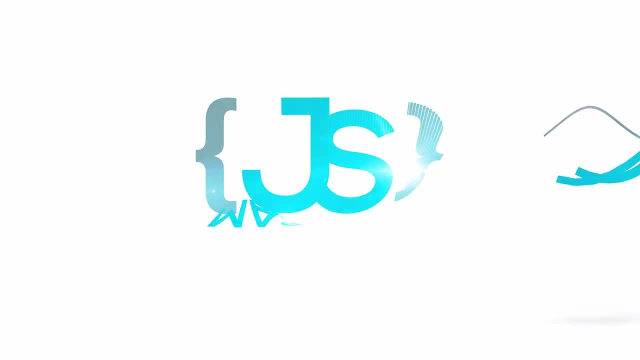 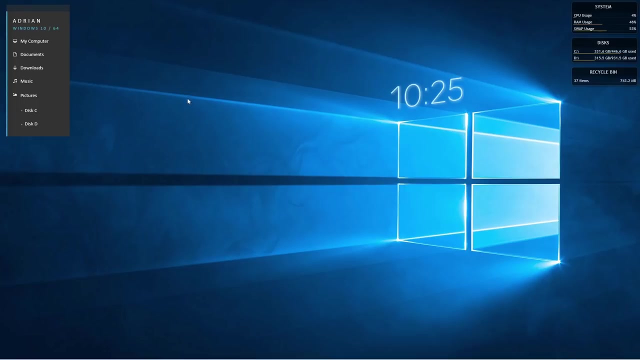 through the process of learning Material UI. With that said, let's start creating our Material UI project. As always, start off by creating a new empty folder. Let's call it something like Material UI Demo. Then you can open your code editor of choice. In this case, I'll be using Visual Studio Code. 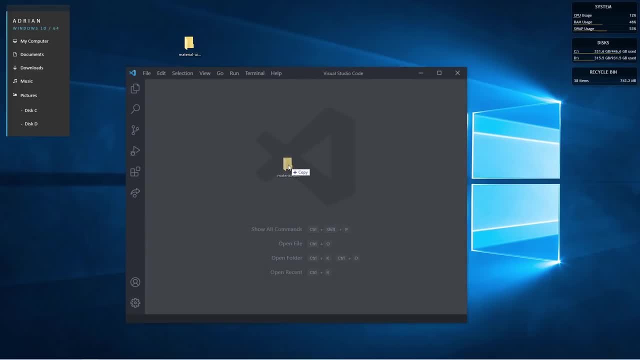 The only thing that you have to do is drag and drop your empty folder into Visual Studio Code. Once that is done, you can open the terminal by going to view and then terminal right here. In this case, we want to initialize an empty folder to create a new Material UI. To do this, we need to create a folder for our 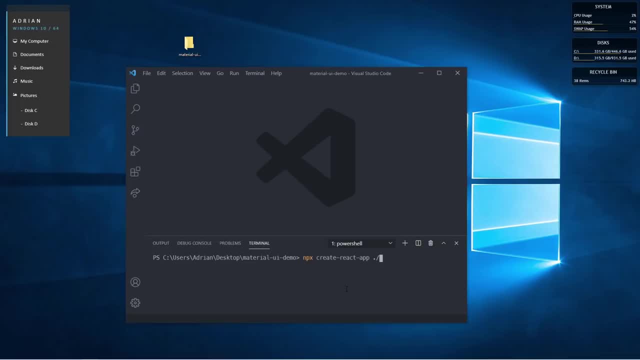 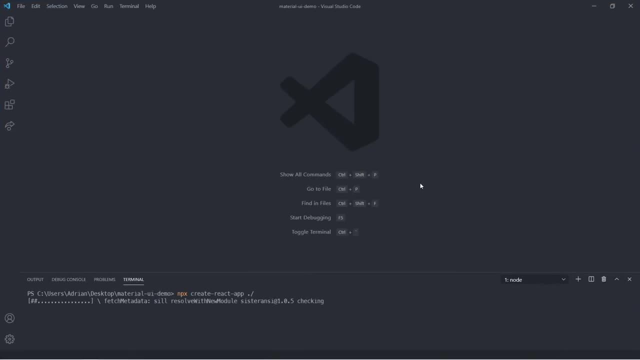 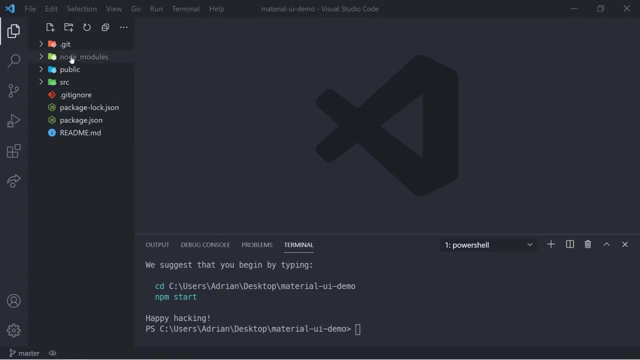 React application. You can do so by typing mpx- create-react-app and then just do /, because we want to create it in the current directory. After you do that, we're going to wait about a minute and we'll be right back Once your React application is initialized. you'll see that a lot. 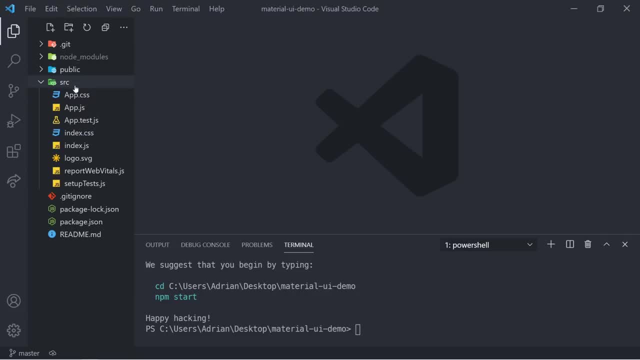 of files and folders have been created for you. The most important folder here is going to be the source folder that we're not going to need, So what I always like to do is simply delete it and create a new one from scratch. Inside of the source folder, we absolutely need to have a file called indexjs. 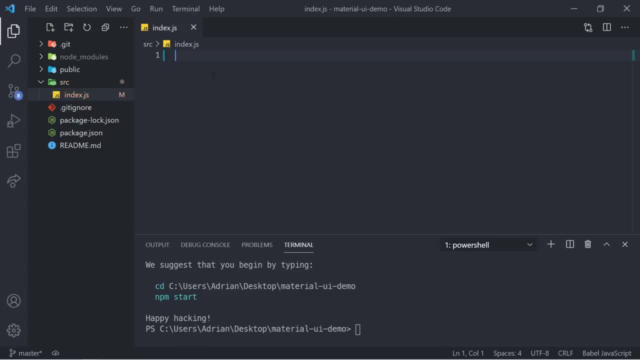 So let's go ahead and create it Inside of the indexjs. we need to import react from react And we also need to import react Dom from react dash Dom. Okay, now that we have react Dom, you can say react Dom, dot render. In here we need to render some sort of a component, So let's call. 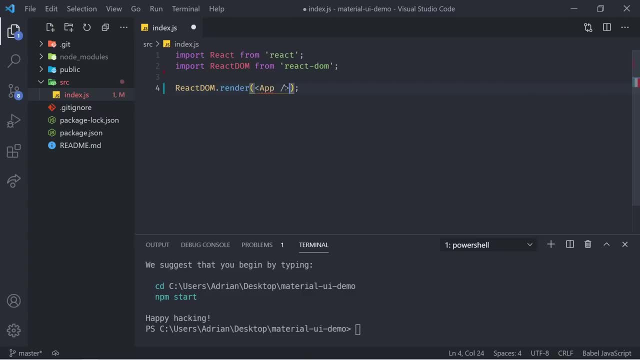 it an app component. This is going to be the main component of this app And you're going to render that to the DOM. Then we have to provide a document dot, get element by ID And then we need to say root. So what is happening here is you're saying I want to render the app component. 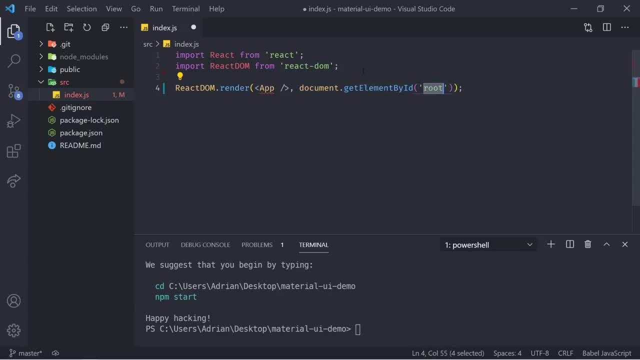 right inside of this root div. that react provides us with. As you can see, app is still not defined, So let's do that. In the source folder, you can create a new file and we're going to call it app dot JSX. This is where our component is going to be. But first, before we create that component, 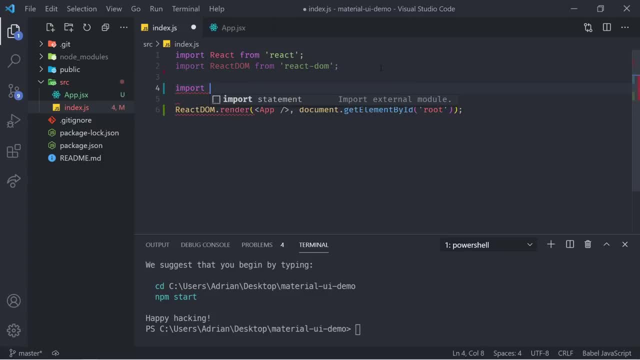 let's just import that app into our indexjs file. you can say import app from dot slash app And that is going to be it for this file. you always need to have one file in your react application where you have the react. 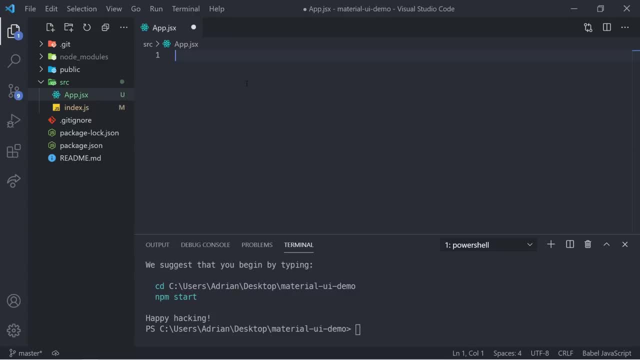 DOM and then react DOM dot render. In this file. For now we're going to create a simple react component: import react from react. Now we can create our functional component by saying const app is equal to a functional component And then in there we can have a return statement. 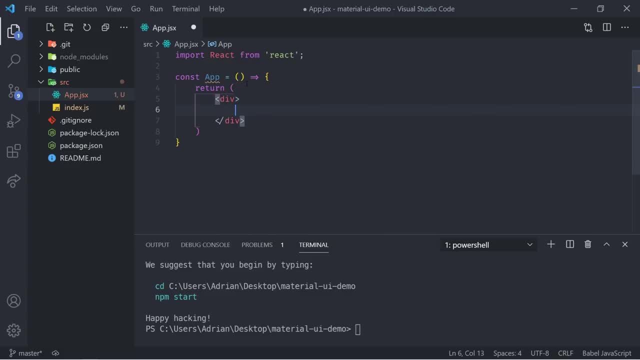 that is, for now, going to return simply a div, And then that div is going to have, let's say, an H one that is going to say hello world. Finally, you have to export default your component. That's it. this by itself should be a functional react component. Before we run it, let's just install. 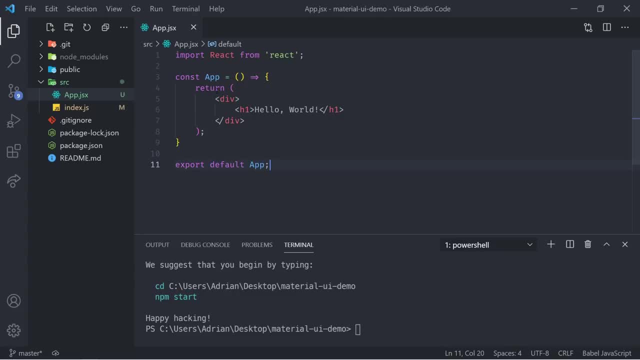 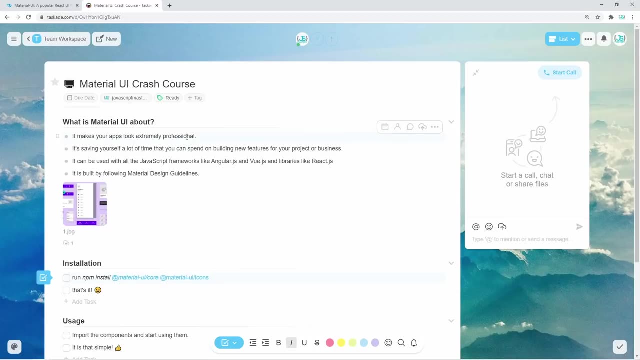 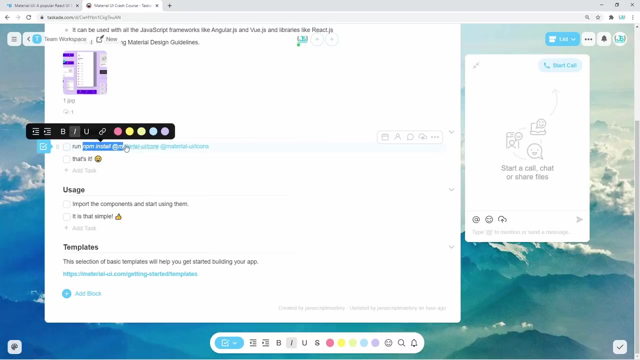 all the necessary dependencies That will need to use our material UI To install material UI into our react application. I'm going to head to the cascade guide I created right for you. As you can see under the installation section, the only thing that you have to do is run npm install at material UI forward. 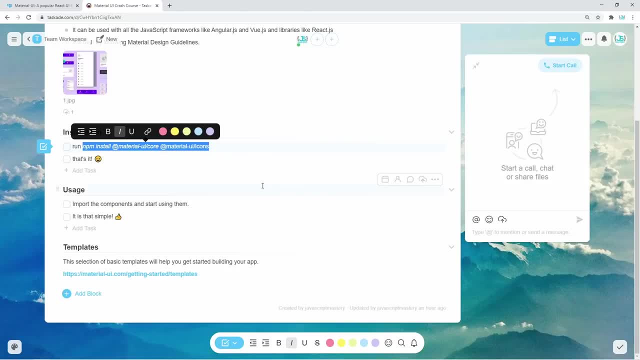 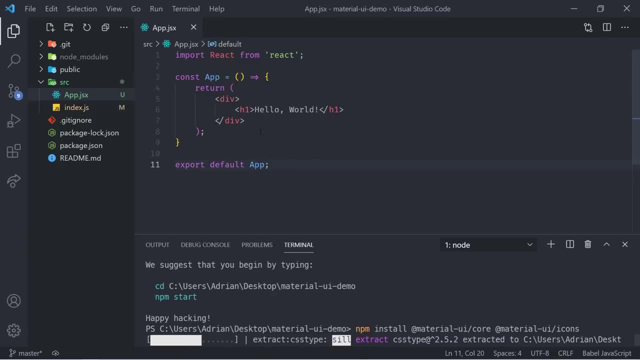 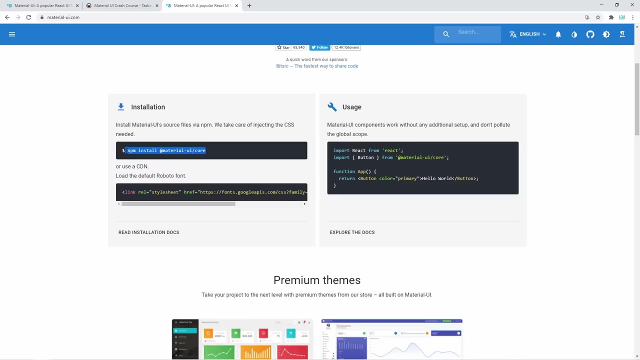 slash core and add material UI forward slash icons. So let's do just that. While this is installing, we can also go to the material UI's website. Inside of here, you can also see the guide to install material UI. we simply need to do this. 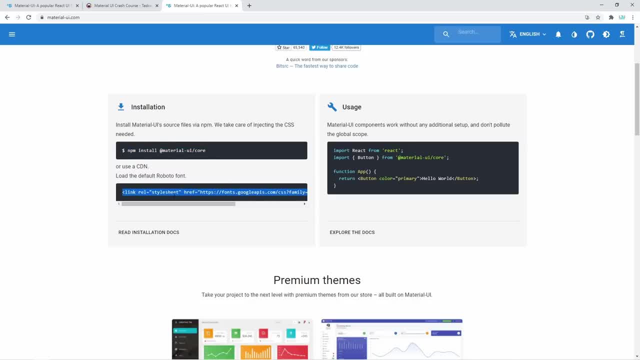 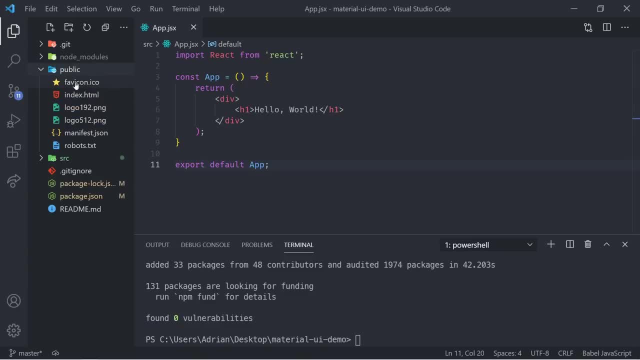 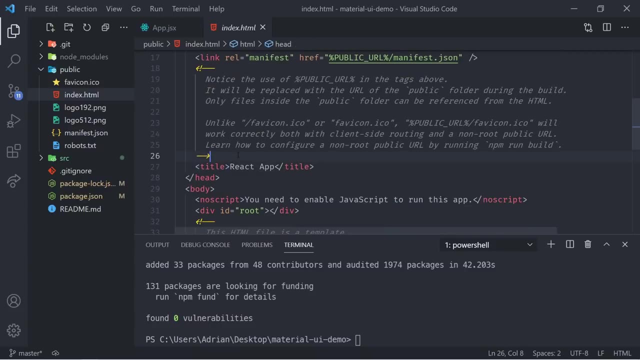 And then you also need to load the font. So let's just copy this line that is on material dash uicom. Go back to our application, go to the public folder and then right into here inside of the index HTML. you can do it just above the title. you can paste that link script right here And with: 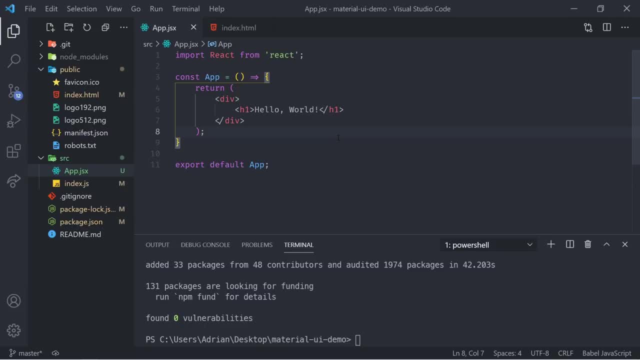 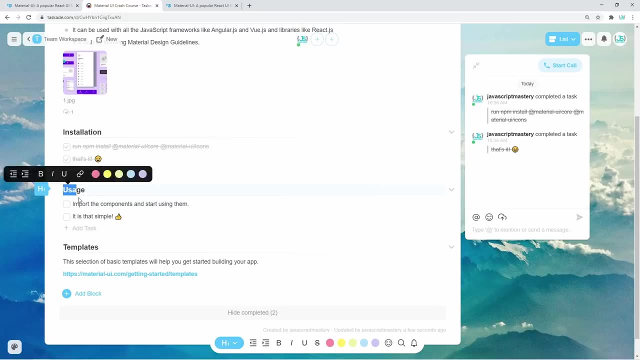 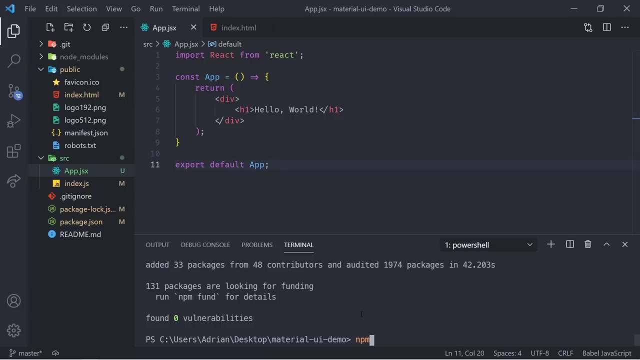 that said, that is it. we've successfully installed material UI. So let's go here And I'm just going to take this as solved. The next step is going to be usage. Let's see how we can actually start using material UI. Back in our application, we can run npm start And that's going to start. 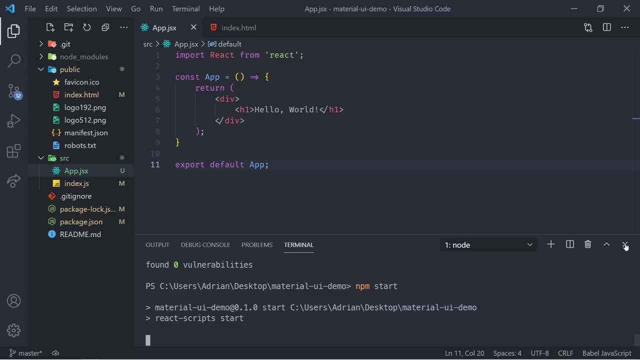 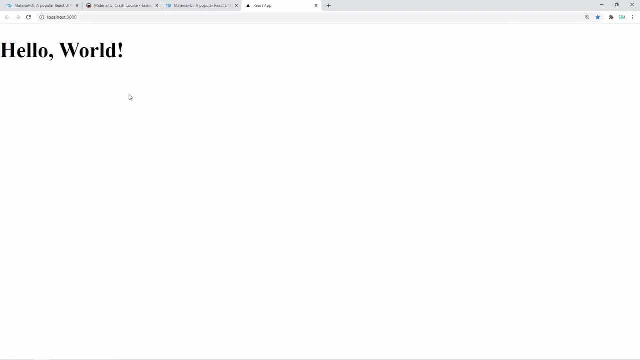 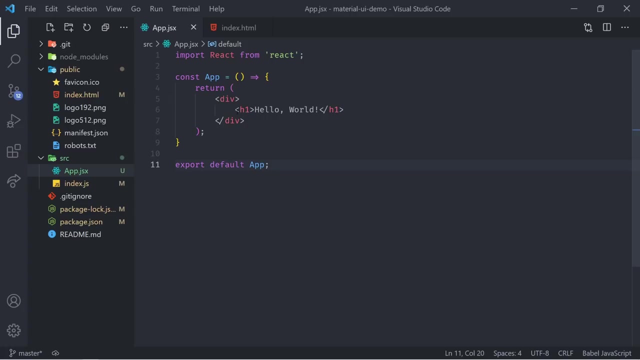 our react application on port localhost 3000.. As you can see, that is it. This is our Hello World application, Just a simple html. Now the question is: how can we start using material UI to make this instantly look better? Well, it is a simple as importing some components from material UI library. you can do that by: 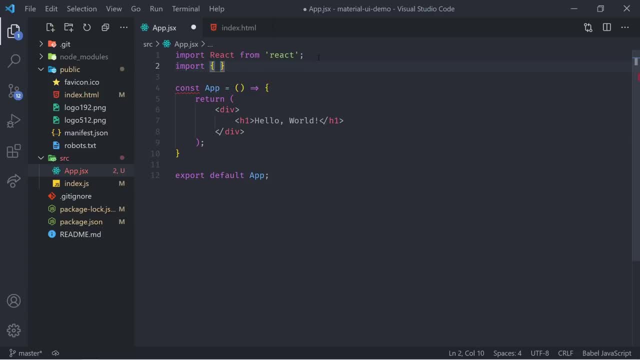 saying import, then you can use curly braces to say that this is a named import, meaning it's not a default one, And you can say from at material UI for slash core. So what components are we going t o import? Well, in this case we can do something like a typography. Typography is a 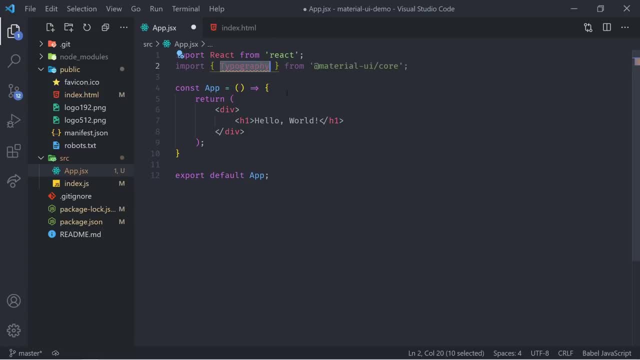 component that you're going to use really, really often in Mat erial UI- Don't be scared by the long wordixes- is just a text. any t extra element is just a text. any text element like a paragraph or a h1, or h2,- anything that you can see as text, that's going to be. a material, UI typography. So now we can change this h1 into typography And then in here you can provide that typeishes to the N? dm candy. If we have a t? p gallery here to be devotional to a N? dmn community, we can write an. 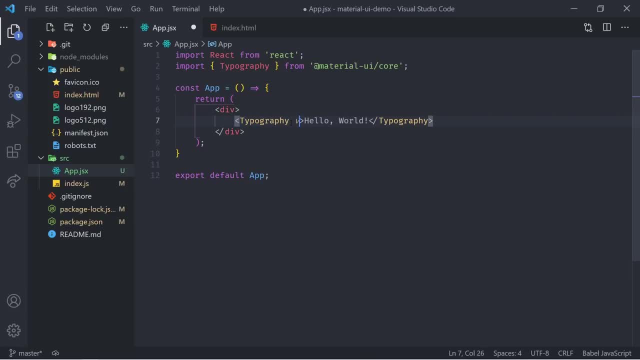 N dmn. I mike as p And unless we're using it as a safeguard, I'm not going to provide any or these things, But remember that they'll be nicer than background0,. npm user: change this h1 into typography and then in here you can provide it a prop, which is a variant we. 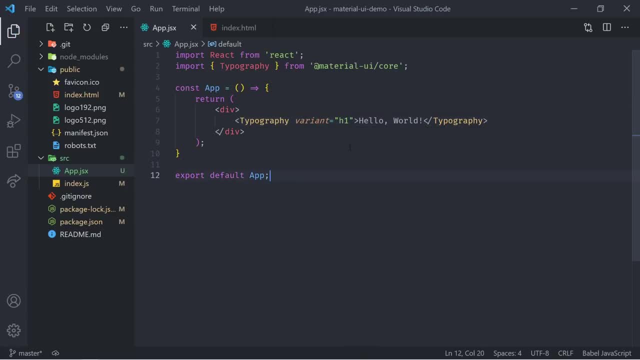 can say variant h1, and right now you can already notice something material ui is going to have these components and it's going to have a lot of different props that can modify those components in a really simple manner. in this case we're saying: we have this typography and the variant. 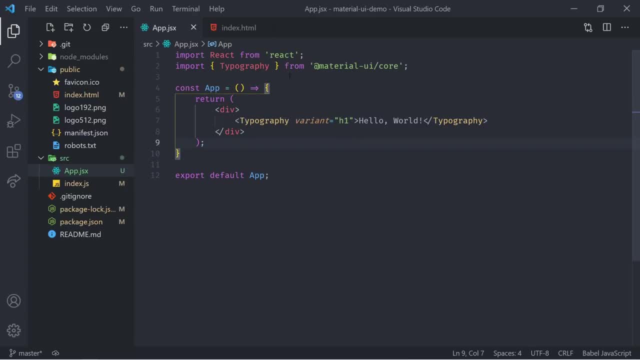 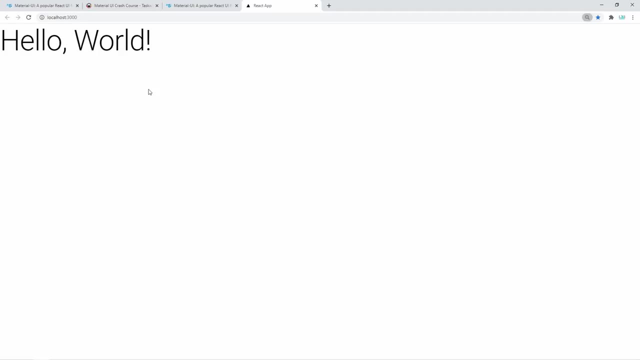 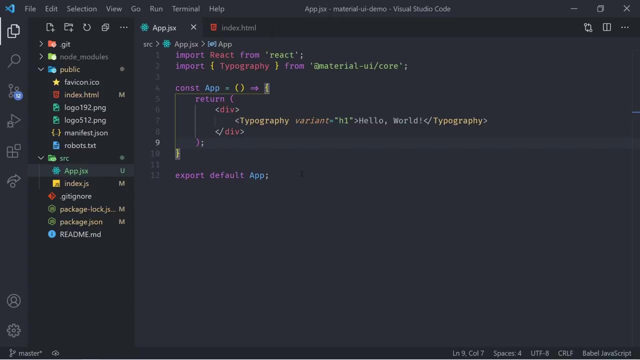 is going to be h1, so let's save this and see how does it look like in the browser. as you can see, it just changed the font a bit and made it look better, but of course, this is still nothing. this is just a simple piece of text, so how can we start using more components all together to make a 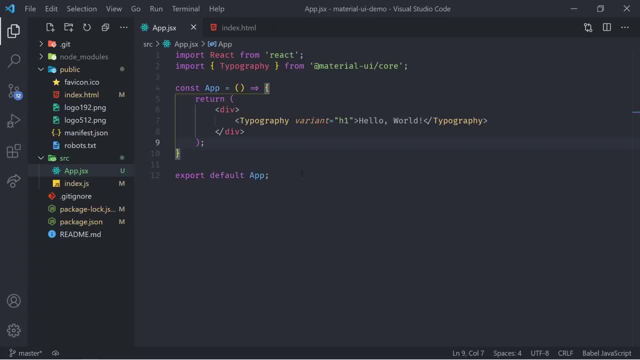 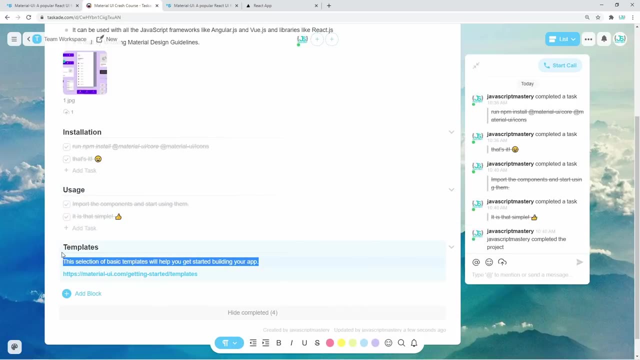 meaningful material design. that's what we're going to do right now. we've just learned how to use components. that's simple, but in this video we're going to go through one of the most popular material you can find in the web, and that's what we're going to do today. we're going to go through 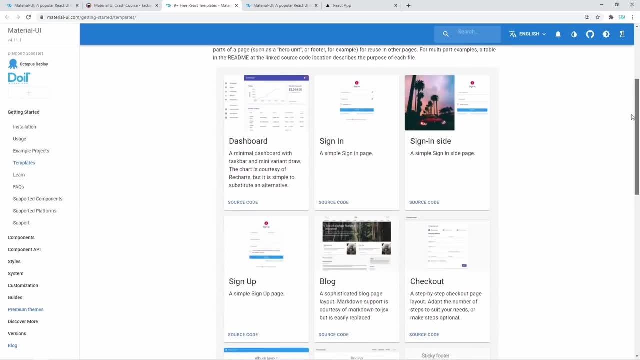 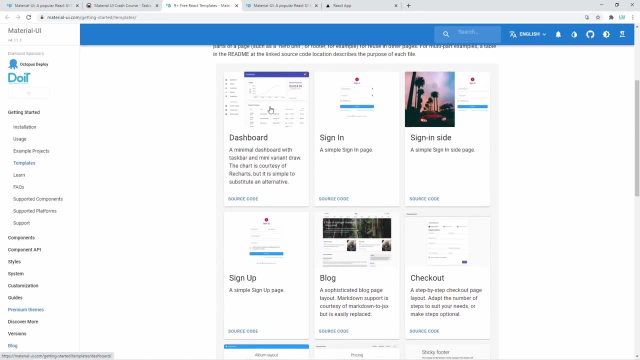 one of the most popular material you can find in the web, and that's what we're going to do today: templates. let's go here and, as you can see, there are a lot of these templates that you can choose from. you can simply copy the code and start using it. for example, we have a dashboard. 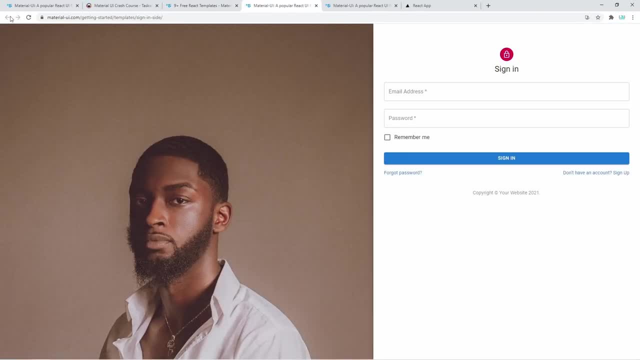 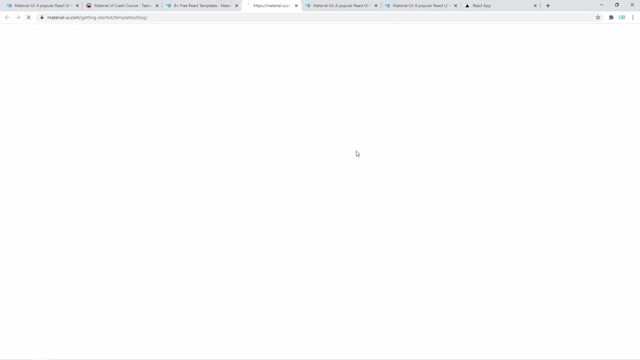 we have a really nice sign in with an image here. we also have a few more nice components that you can immediately copy the code for and start using, for example, this blog right here. that has a lot of interesting things. we also have something like a sticky footer. we also have a. 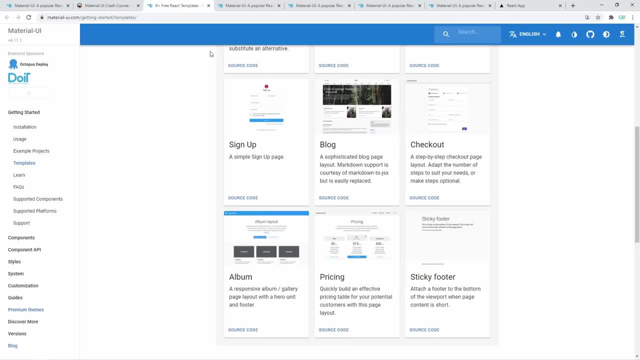 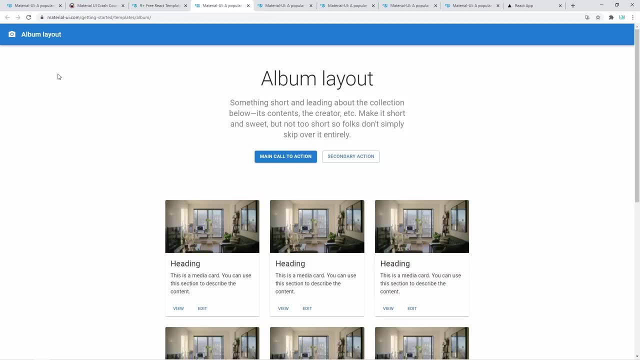 modal for a checkout with a lot of fields. in this case, we're going to use this album one. i'm choosing to use this one because it nicely covers most of the things that you need to know to learn material ui. we have a header. every application has a header. we have a nice hero. 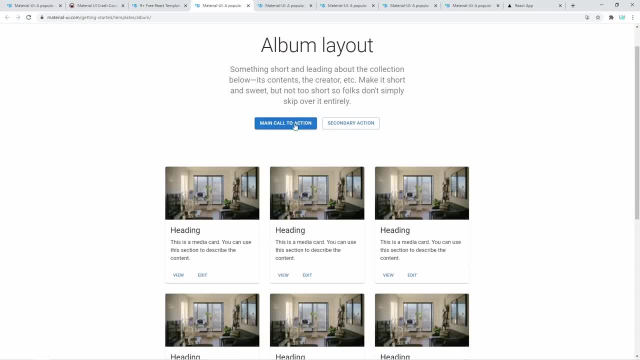 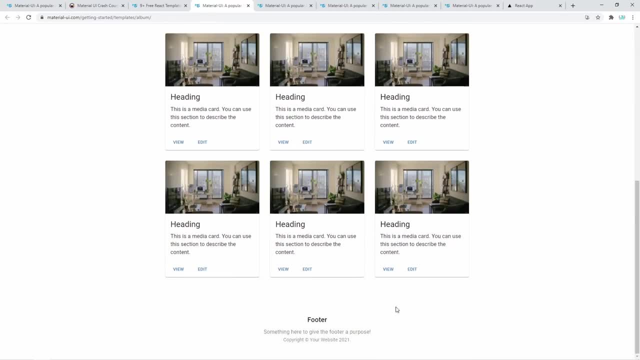 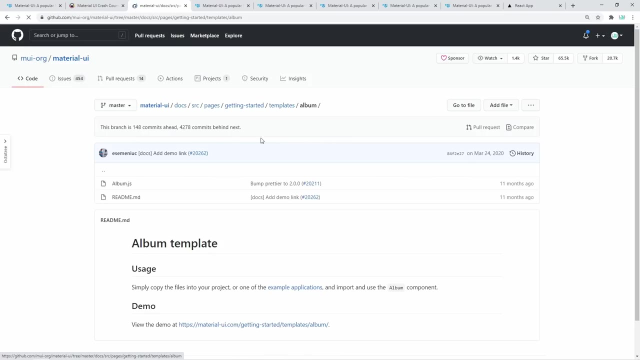 section with an h1 and some text. we have call to action buttons. we also have these cards, which are great for representing data and moving forward. we also have a footer. so in this video, what we are going to do is not simply go here, go to the source code and simply copy the entire. 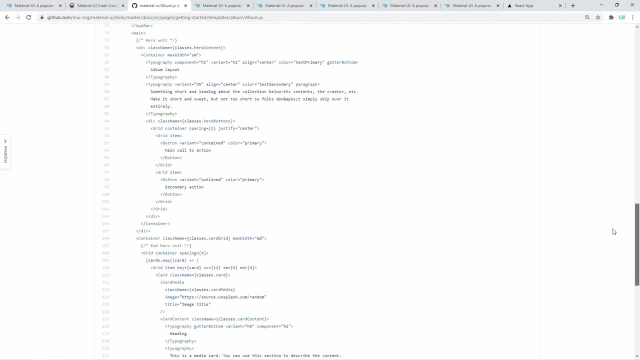 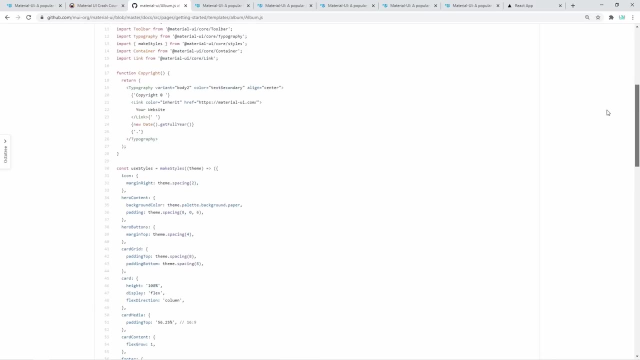 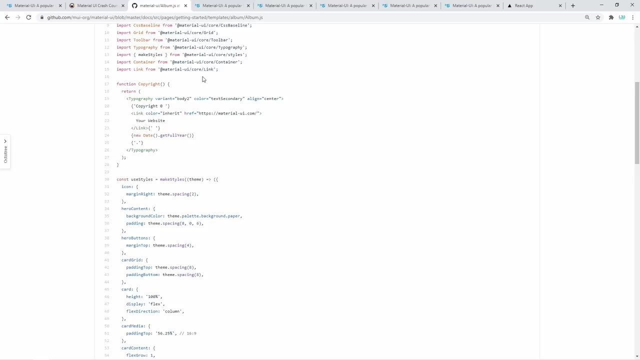 code that we have here. that way, you wouldn't learn anything. what we are going to do is we're going to write this component entirely from scratch, line by line, and i'm going to teach you how to do that, not only how you can watch me and copy that. i'm going to teach you how you can replicate this. 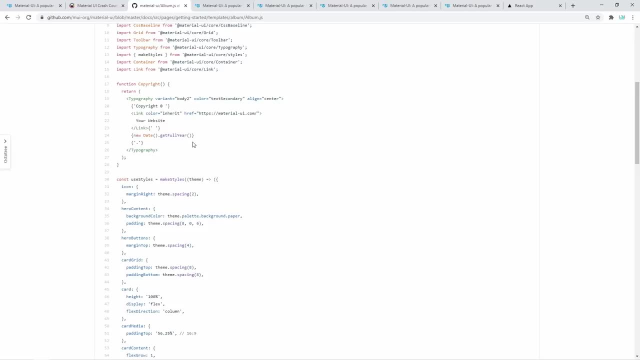 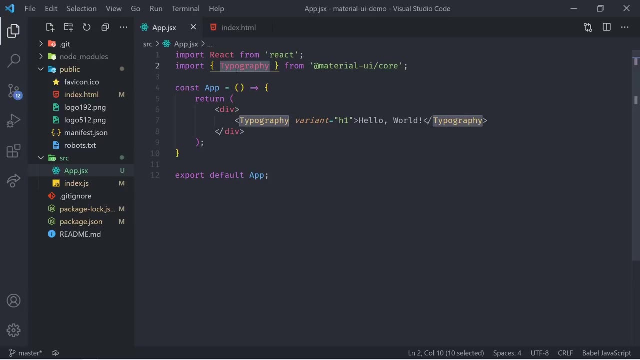 and extend that and build more projects using material ui. so let's get started. in our application, we'll need more components than a simple typography, so let's import all these components right now. first is going to be the typography, then we're going to have the app bar, which is going to be that navigation bar. we need card as well as the 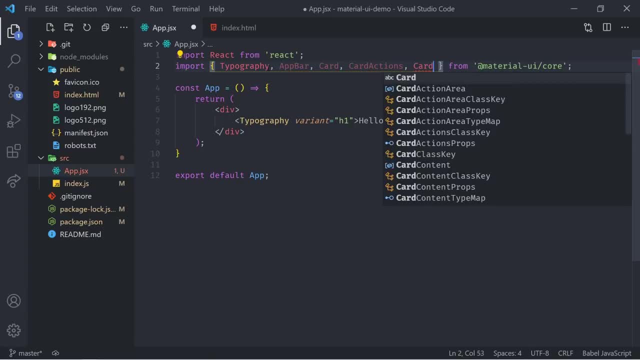 card actions and also card content. we also need card media. alongside that, we're going to need a ss baseline that's going to immediately provide some styling for our application. next, we need a grid. we're going to use a grid for responsive design and positioning. then we have a toolbar, we'll have a typography and finally, we're going to have 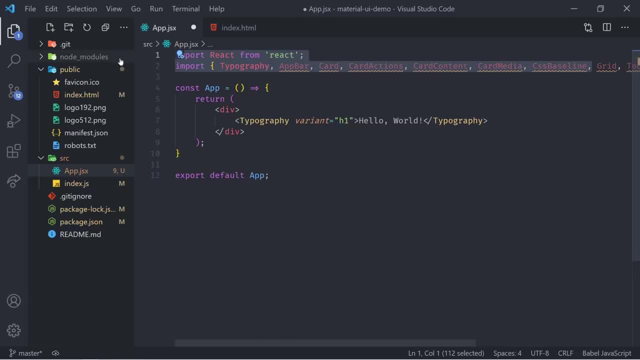 a container. these are all the components that we need. as you can see, it's quite a long list, but in this video, i'm going to teach you how to use them. we're going to also need an icon for our navigation bar, considering that we're building some sort of a photo album. 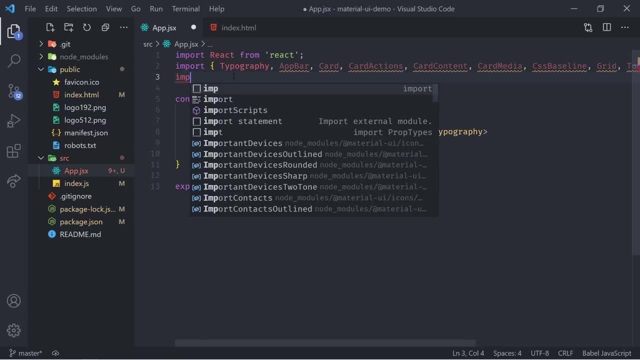 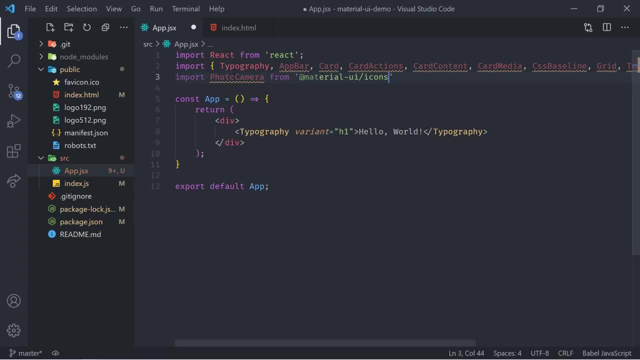 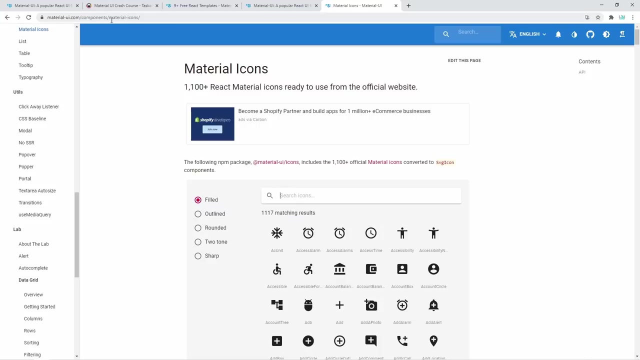 we'll use a camera icon. and how can you do that? well, you can simply say: import photo camera from. add material ui forward slash icons- great, in case you want to see what icons are available, you can head to material ui components and then icons and then in here. 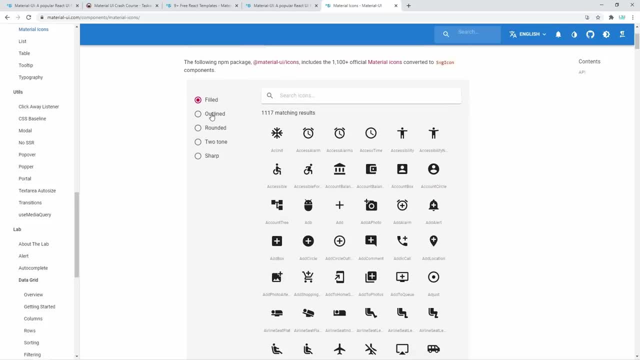 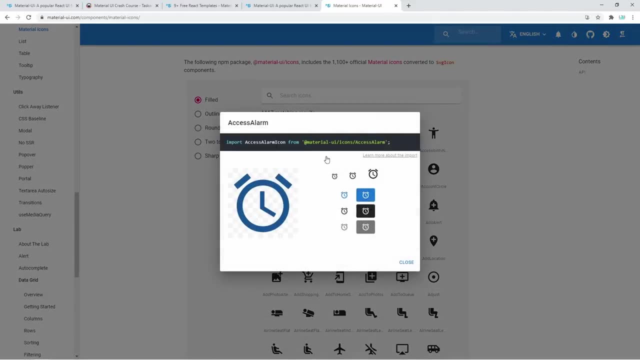 you can search from 1000 different icons. you can have them as outlined here. i'm going to select simulation Lincoln from the miidos and then from there I'm going to select point-based proportions. so this is going to be the important thing there. we're going to 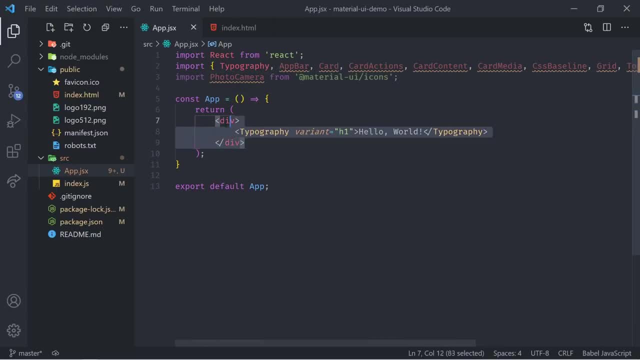 put writer icons here and let's drag and drop. write that up a little bit for you. turned this Lightroom in in the whatever is cálculo mode, like minimum acabar, and always comes back to normal. if us very high setting, we're gonna start using this module to always. 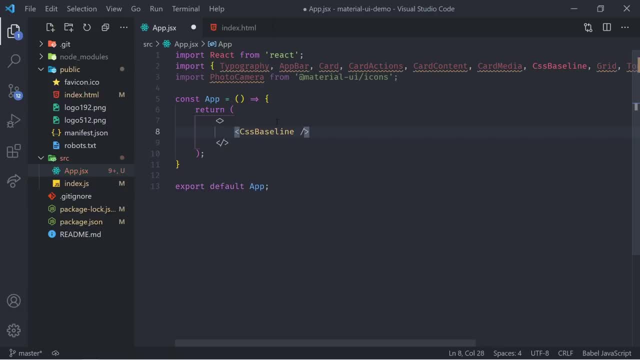 make sure that the display is important and that we have right up here to think that the frame of the picture is gonna be the same concept as the Coll臺 to be exact. so this code will take quite some time, says baseline. here is going to provide a lot of default styling for your material UI applications. 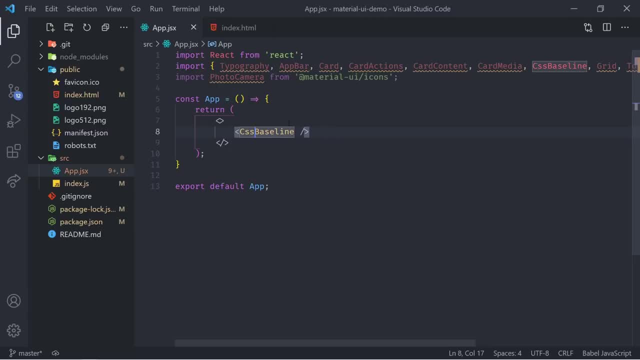 so that you don't have to worry about the styles. As soon as I add a few more components, you'll start noticing the difference. The first thing below that is going to be the app bar. App bar is simply our navigation bar. It is going to have a position of relative Inside of there. we're also 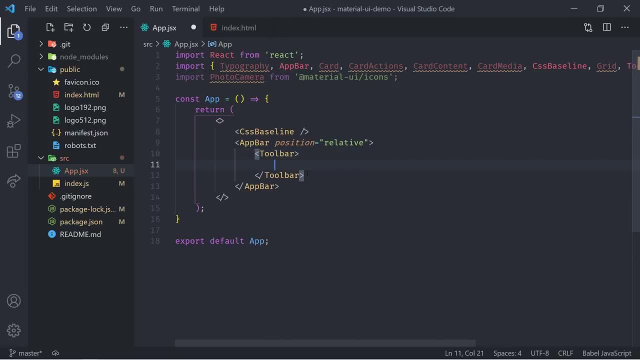 going to have a toolbar. Toolbar is that blue line. you'll be able to see it really soon. Inside of toolbar, we'll first have the icon. The only thing that you have to do to include that icon is simply putting it right there. That is it. Finally, next to the icon, we're going to have a. 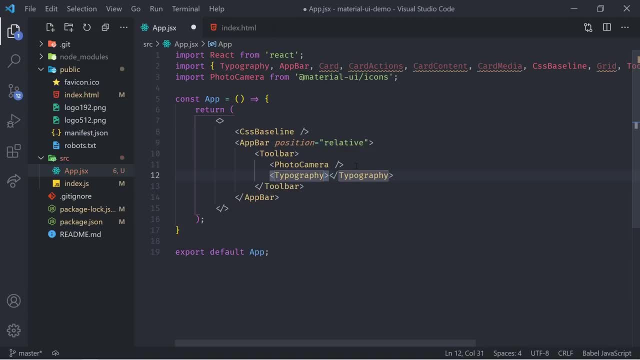 typography. We already learned what that is. That is simply a piece of text. In this case, we're going to have a variant that is going to be equal to h6.. Inside of the typography, you can type the text that you want to use. In this case, let's say something like photo. 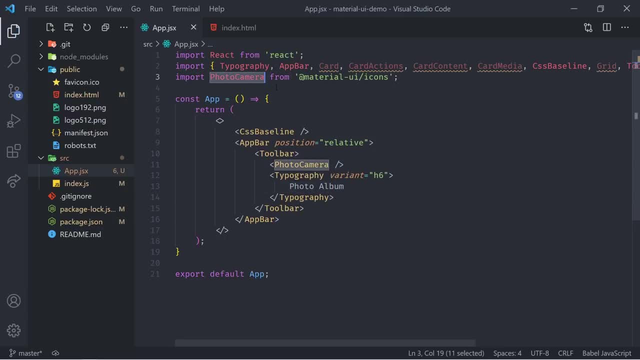 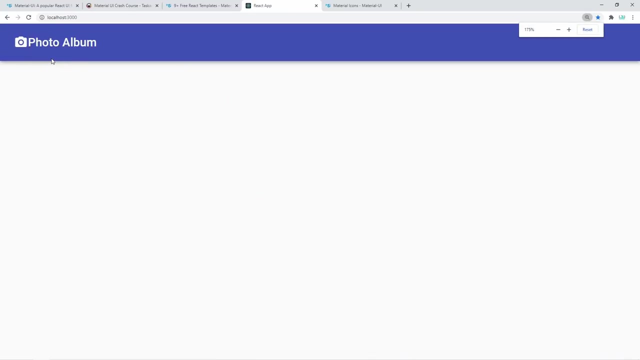 Just before we test it out, I noticed that this here shouldn't been a default import. We also needed to put curly braces around it. With this done, what do you think? What are we going to see if we check our website? Well, take a look at that. We already have this nice looking navigation bar. 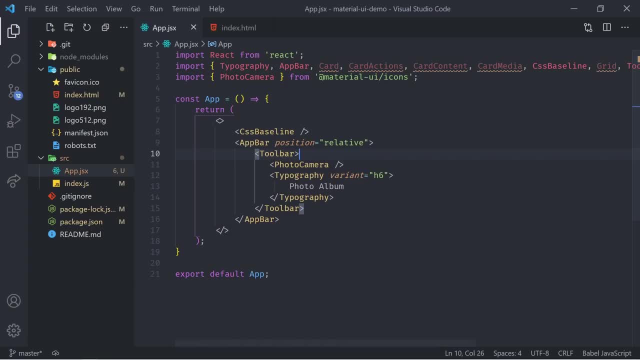 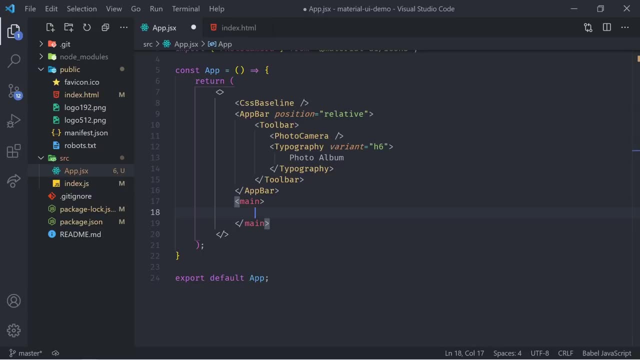 at the top. Great. so now let's continue on to our main part of the application. We're going to use semantic html tags like main, to indicate that we are now on the main part of the application. Inside of there, we're going to create a div, and then, inside of that div, we're going to create a. 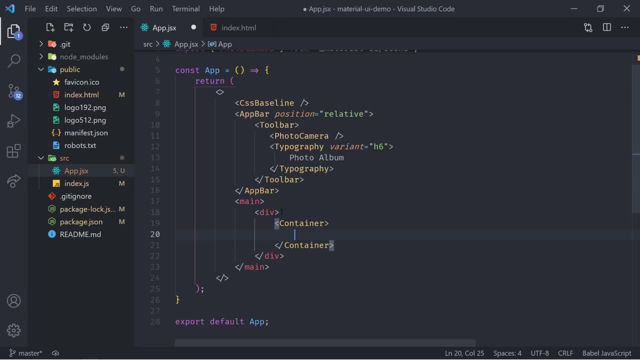 material ui container. Container is basically as the word sounds. it contains different things inside of a specific area of the page. This container is going to have a max width of small sm, for short. Now we're going to put something into it and then we'll see. how does it look like? 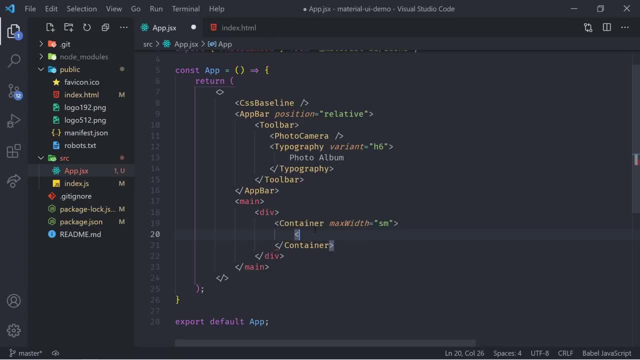 First thing that we're going to put in, there is going to be a typography, So I'm going to put a typography right there. This typography is going to have a variant of- let's do- h2.. It's going to have a property, align, which is going to be set to center and the color is going. 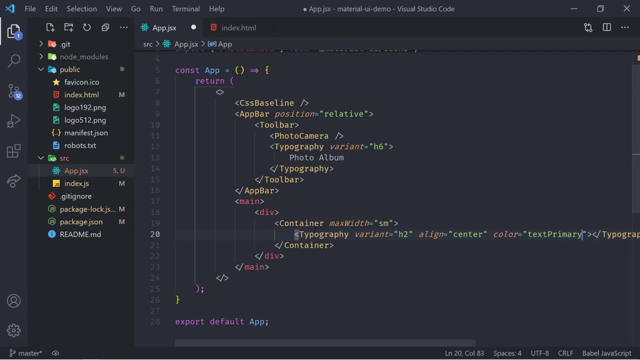 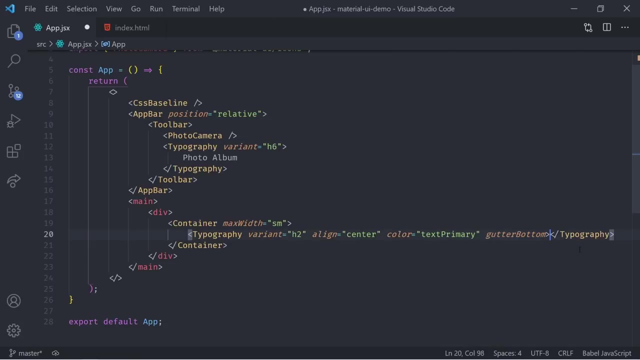 to be equal to text primary. These are all properties that material ui allows you to have. We're also going to add one more property, which is called gutter bottom. This simply is going to add some margin To the bottom of this specific typography. Now, in there, let's type something like: again, let's do. 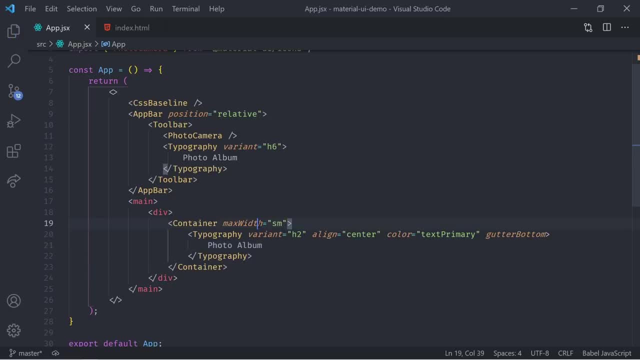 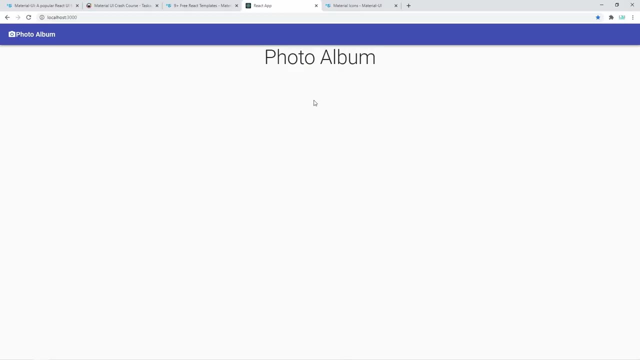 photo album- Great. So if we save that, let's see how does it look like. As you can see, we already have this nice heading at the start. Of course, later on we'll have to style it a bit, add some margin and make it look nice in the center of the page. Now let's add one more: typography. 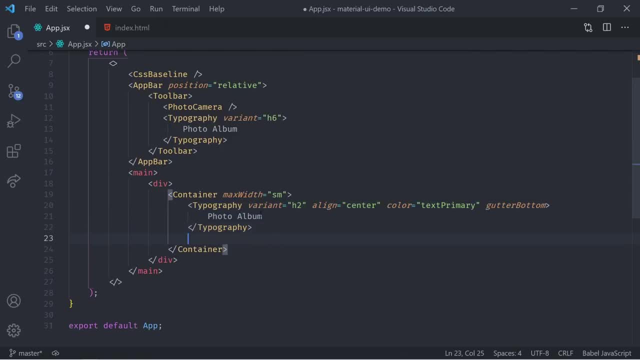 This one was a heading Simply saying what page we're on, But the second one we're going to add right now is going to be the explanation of what people are going to see on this page. Again, let's do a variant This time. 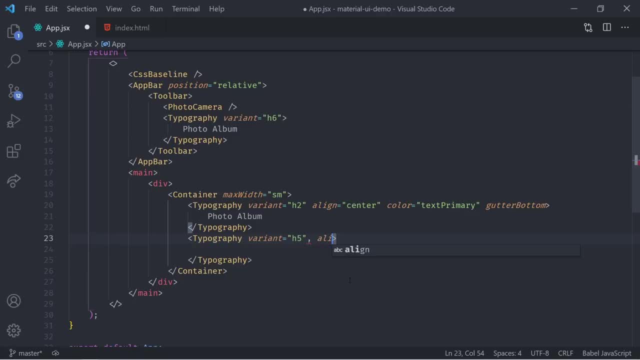 we can use something like h5, a bit smaller. We'll again use the align, which is going to be set to center, And this time the color is going to be of text, secondary Nice, And we can also provide a paragraph. This is going to make sure that it looks like a paragraph, So we're going to add a. 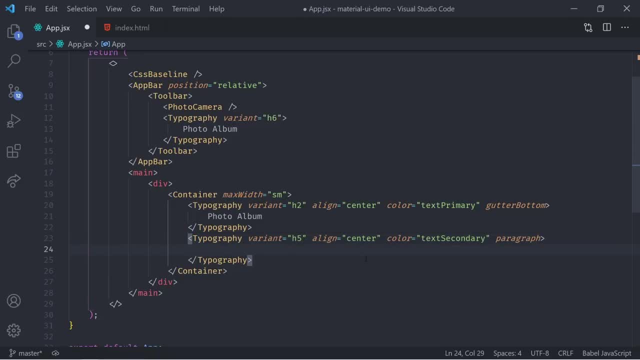 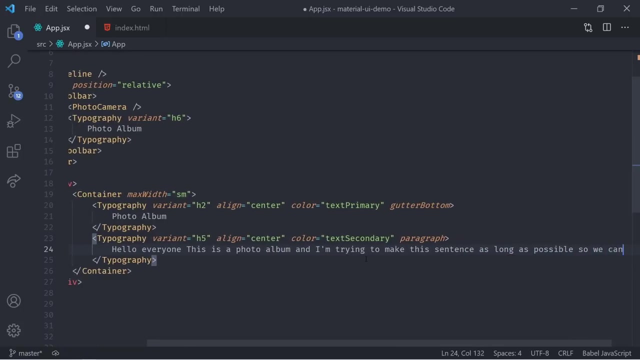 paragraph that loops through the lines Inside of this typography. let's have a longer paragraph, just so we can see how is it going to look like on the page. Let's do something like: hello everyone, This is a photo album and I'm trying to make this sentence as long as possible so we can see how does. 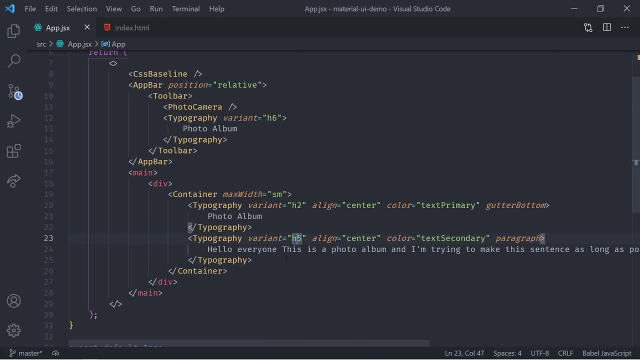 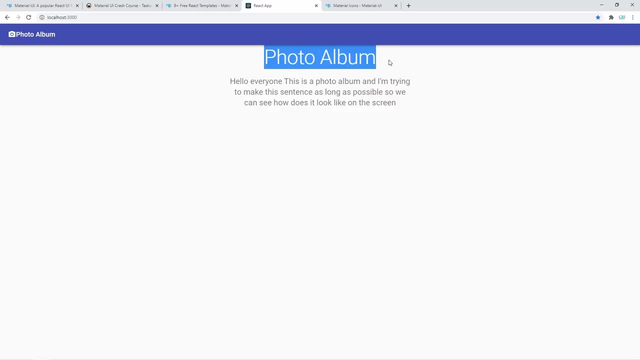 it look like on the screen, Great. So this is going to look like a paragraph And we're going to add a paragraph that loops through the lines. This is a long sentence that I just made up, and let's see. how does it look like. As you can see, we have this primary text and we also have this secondary text. 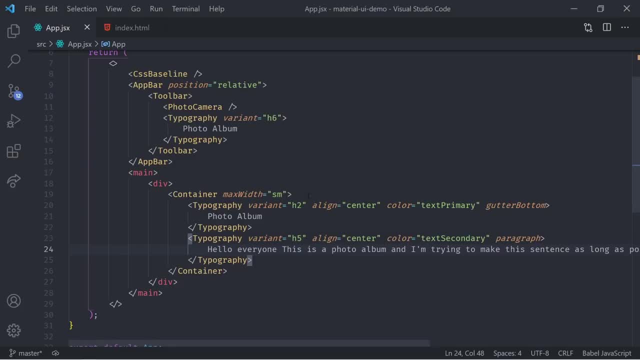 right there. But you might be wondering how did I know to put this variant h2 here? How did I know to put this max width small here? How did I know to put the align color gutter paragraph or anything else that you can use as a prop to material UI components? 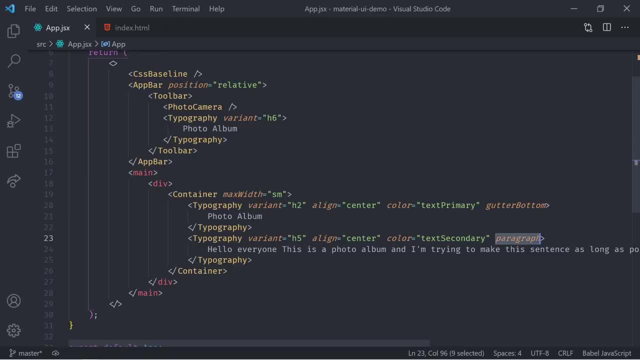 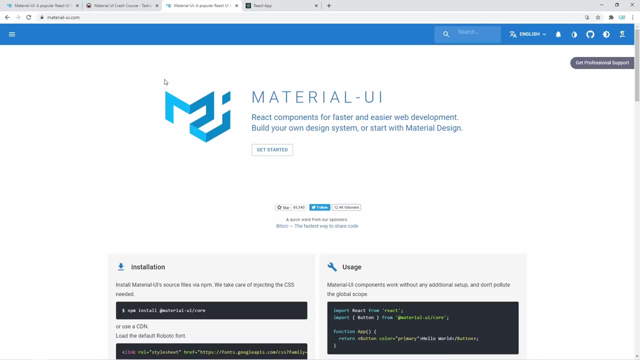 is the main question. I don't want you to simply remember these four or five different props. I want you to understand where you can find and learn more of these props, and that's exactly what you're going to learn right now. On the Material UI site, click the upper left menu and you'll see a sidebar. We're 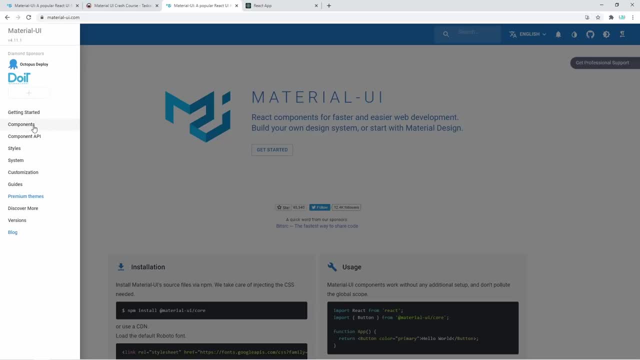 first going to talk about two sections: components and the components API. The main difference between these two sections is that the component sections contains examples, demos and explanations for each component. Let's take a look, As you can see. if you expand it, you can see that we have demos and explanations for. 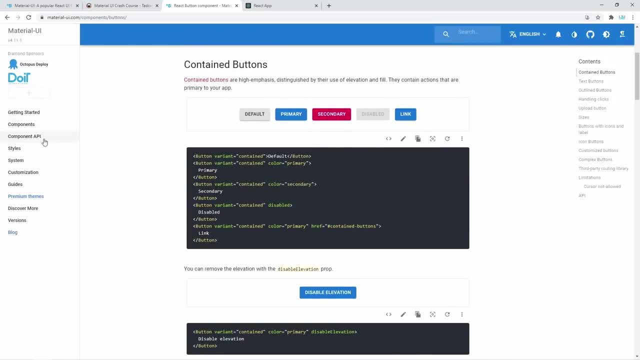 each specific component. On the other hand, the components API contains a complete list of props and CSS rules classes for each component and no examples. Each component appears in the both sections, creating a nice separation between the exploration and checking exact property names. So how would you go about researching this? Let's say that 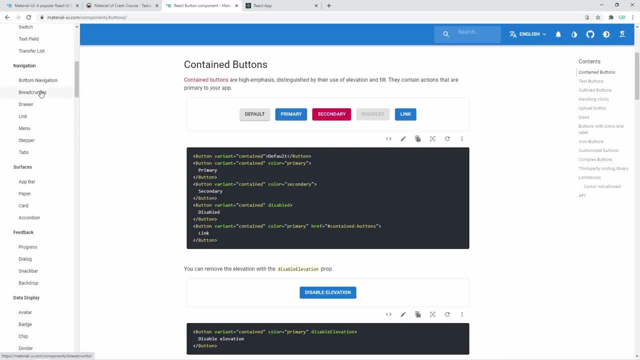 you want to use a typography, the one that we just used- You would first go to the component section and then in here you would find a typography. You can also just search on the right top side. So in here, typography components, In here you. 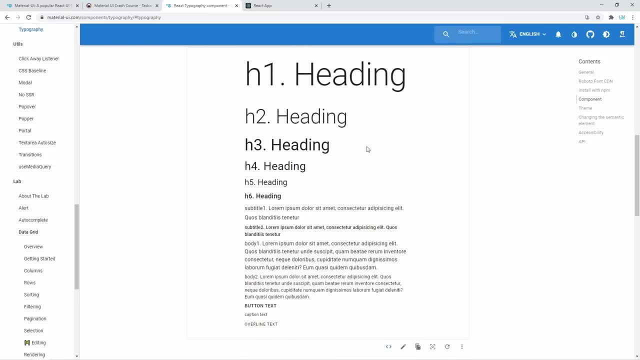 can see what components can you use and how you can achieve this. look, The component section is where you are going to spend most of your time when researching how to use Material UI. The most important part about each component is that there is actually working examples on the page that you can try out For. 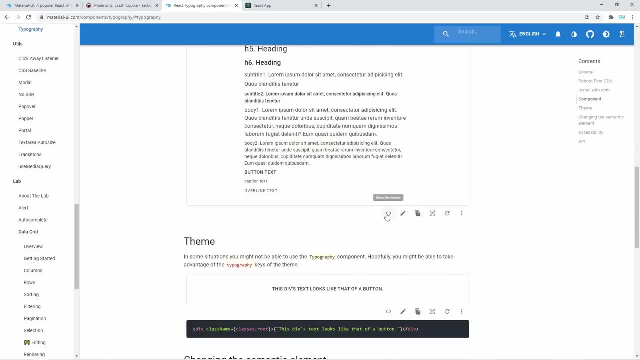 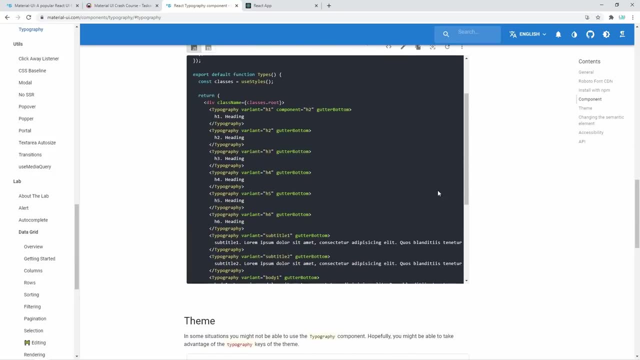 example, you can see the full source code by pressing this icon right here: Show the source. When you click that, you'll be able to see the entire code to reproduce what you just saw right in here. Best of all is the component section is the highest valueost ien, so this engagement part doesn't work out too well. 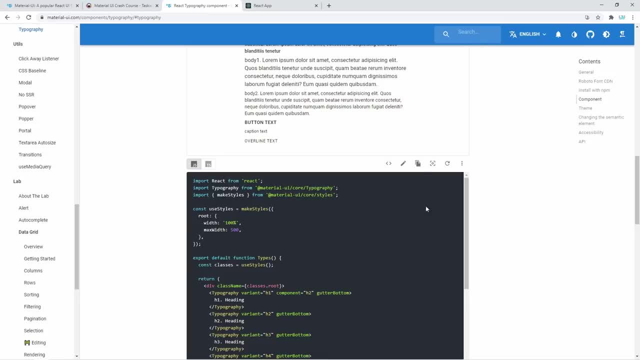 These examples actually work, so you can simply copy and paste the full code into your project and that's it. you'll have it right there. Let's not take the typography. let's take something that we haven't used so far, something more complex, for example. 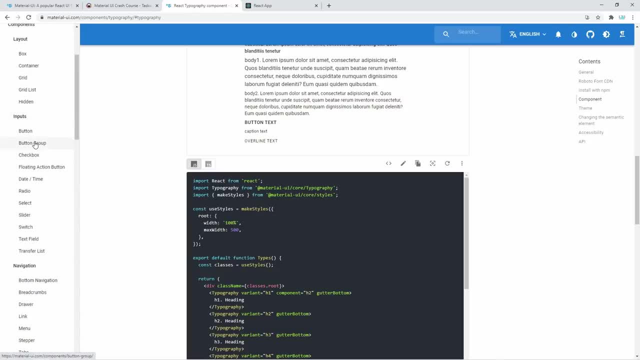 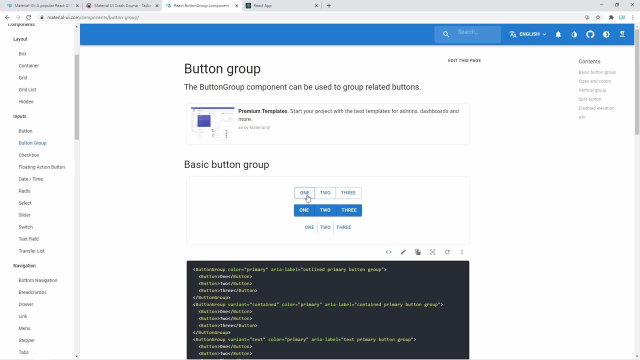 So, if we go into the components, let's try taking a button group, for example. As you can see, this is a group of a few buttons. to actually create this using normal CSS it would take some time, but in here you have it really, really simply. 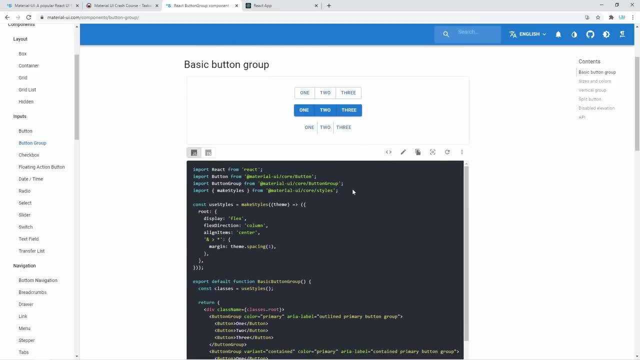 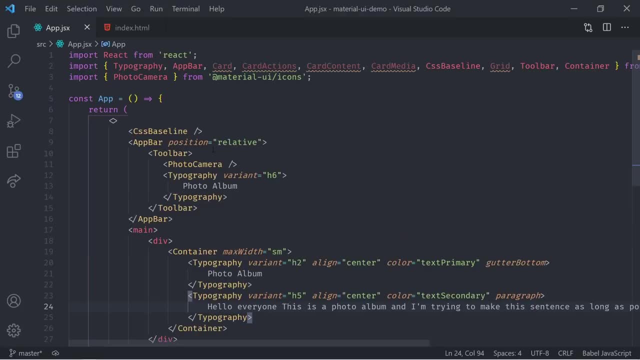 So you can click show the full source. then you need to import some things. in this case I'm going to import the button and the button group so you can head back to the project. we're first going to copy that part right in here and then you can simply scroll down. 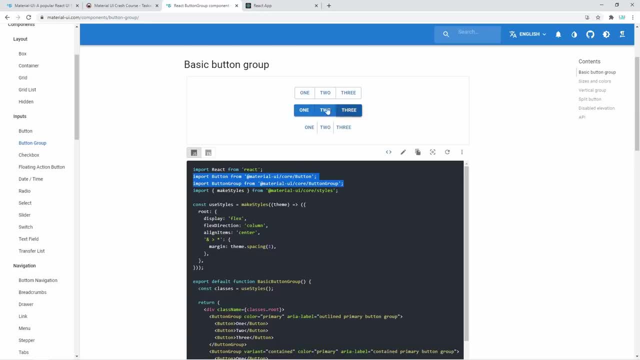 and you can take the example that you want. For example, I'll take the second one, and that is going to be this one. here, I'm going to take the second one, and that is going to be this one. here, I'm going to take the second one, and that is going to be this one. here. 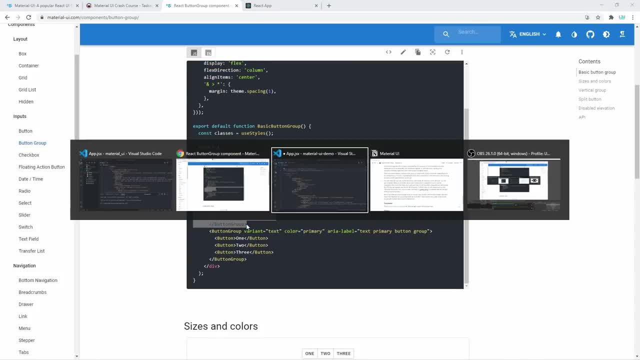 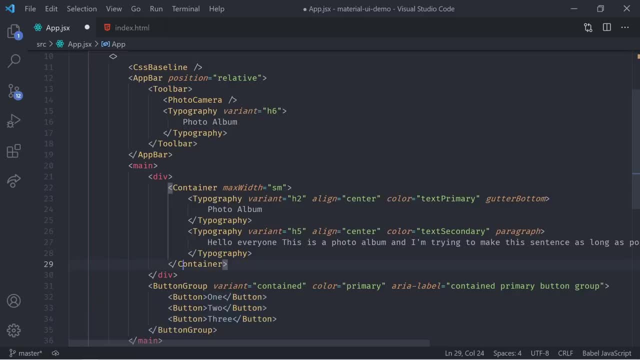 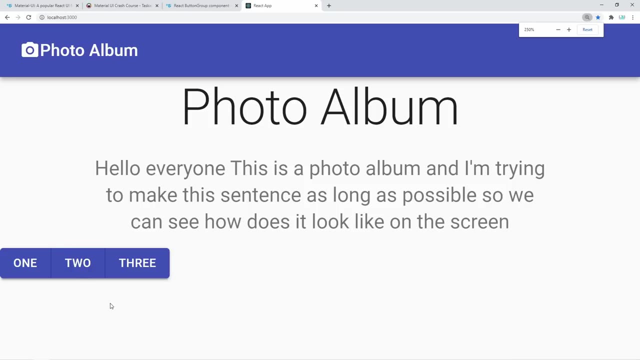 I'm going to copy this button group and simply paste it right inside of my application. Let's do it just below this div right here. I'm going to indent this properly and save the file. If I go back to the application, as you can see, right on the left side we have this: 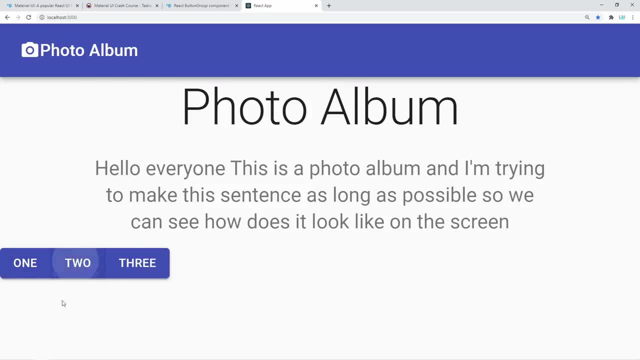 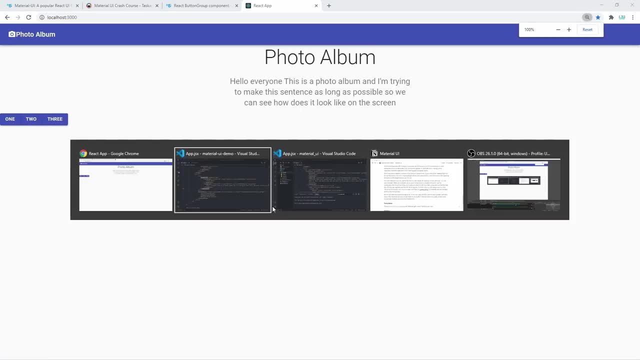 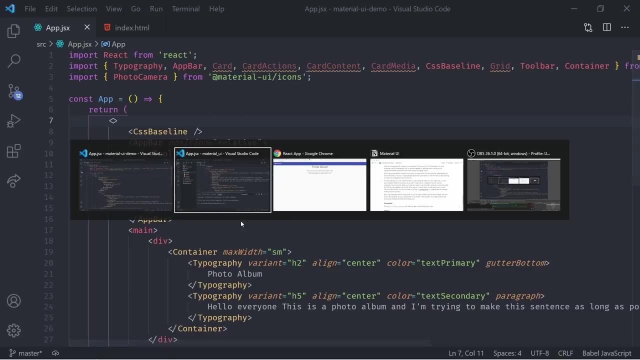 button group right here looks nice, has the hover effects, has the click effects and you can simply start adding the logic. This is the power of Material UI For now. let's get rid of this. let's get rid of the imports as well, and let's focus on the things. 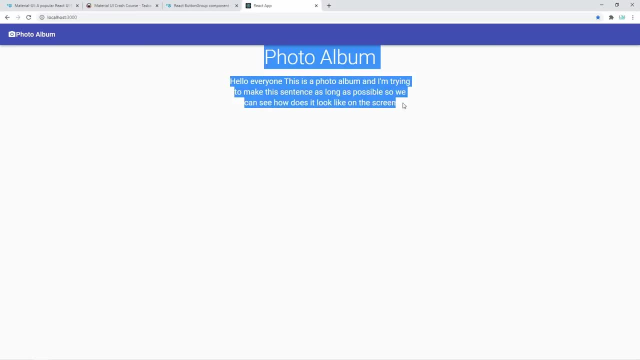 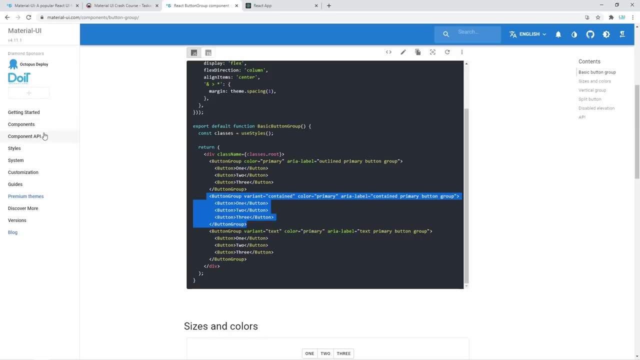 that we actually used already. These are going to be typographies For the typography. you don't want to simply go to the components and then typography. you want to go to the components- API, and then you need to find the typography right in here. 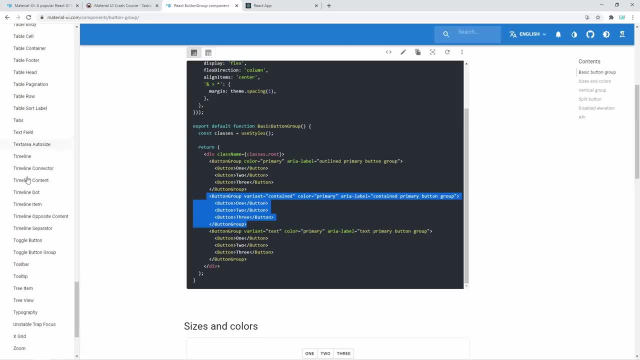 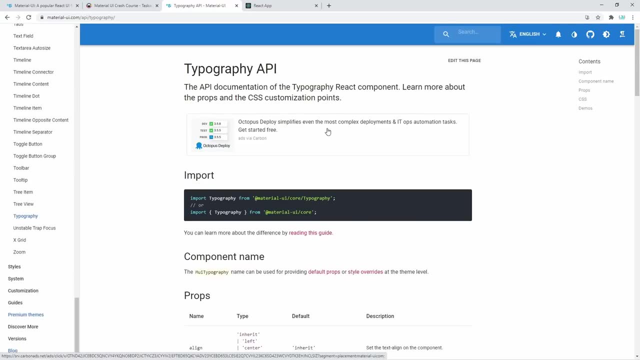 If you just scroll a bit, we can use the search bar on the right side, of course, but let's find it right in here. There we go. This is not the typography component. this is the typography API. Inside of here, you can see the full documentation of all the props that you can put. 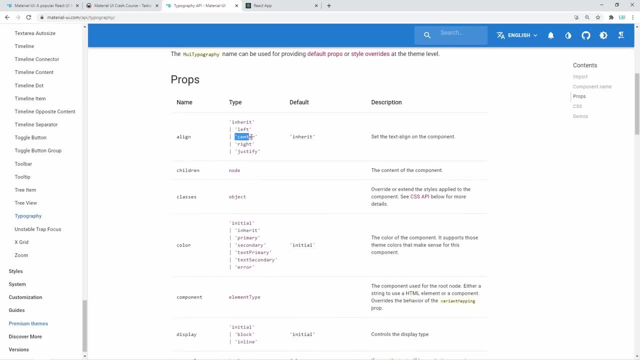 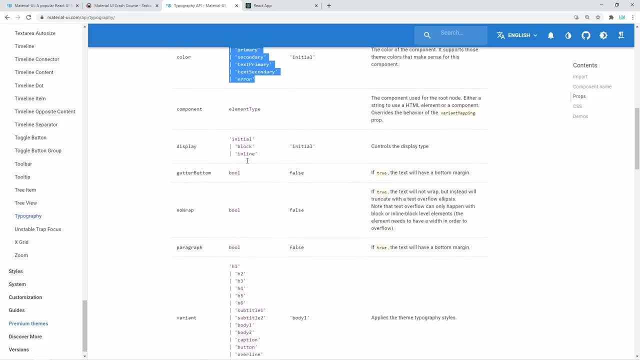 For example, you know that in the code we use the align center. So now that you know you can use the align center, We can also provide some classes. you can see which colors can you choose from. You can, for example, change the display. you can add the bottom margin we also use. 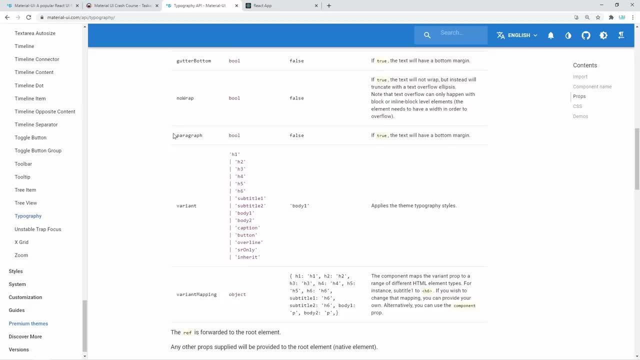 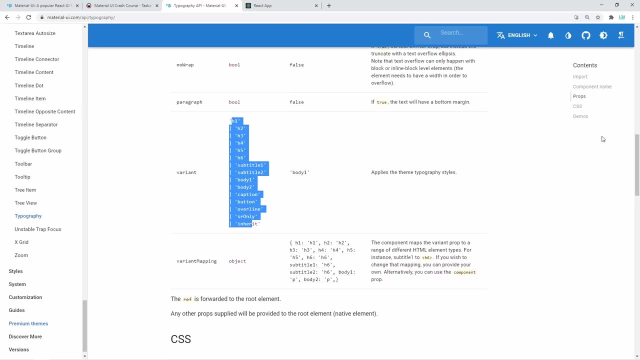 this: If we use paragraph, the bottom will have. if we use the paragraph prop, it's going to have the bottom margin as well. and you can also see all the different variants. This is amazing. This is how you learn how to use any specific package. 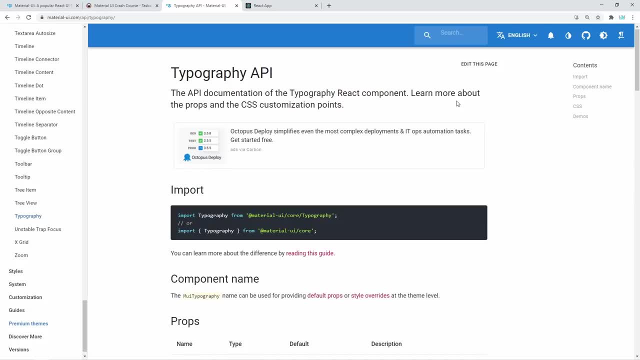 It doesn't have to be Material UI. it can be an NPM package you found online. You need to read the API reference documentation. With that said, now you know how you can find new components that you want to use in your applications in the component section. 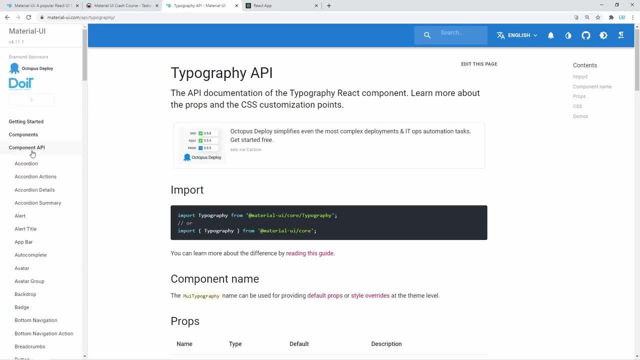 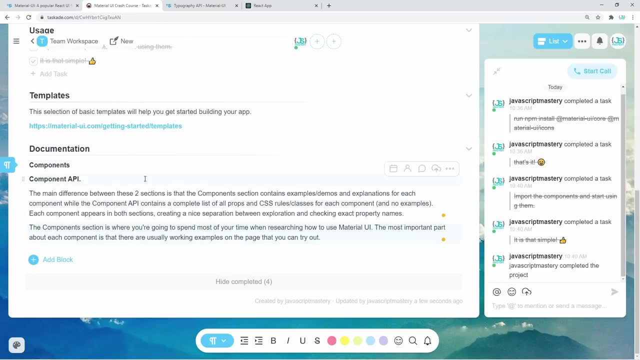 And then, once you start using them, you can read more about them in the components API section. That is amazing. With that, we went through the last part of our Taskade list, But while we're here, I just want to show you a few more features. 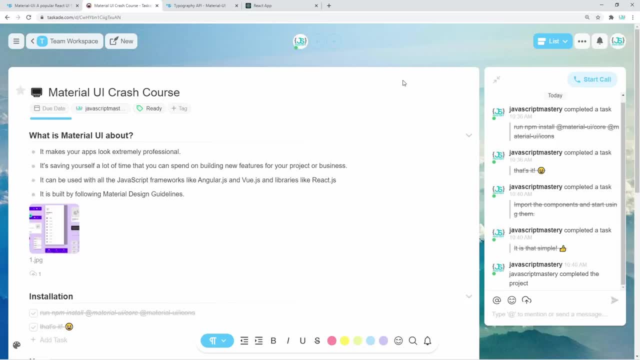 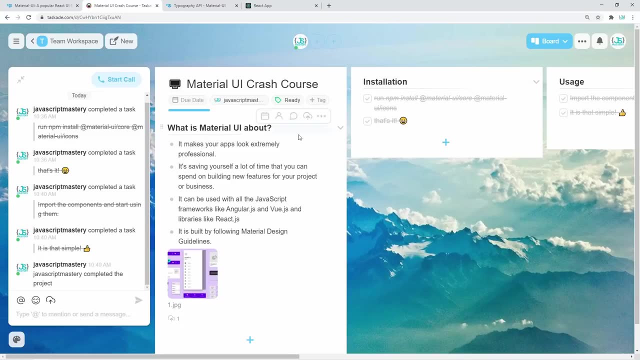 Taskade is amazing for collaboration on different projects. You can invite project managers, developers and everybody can collaborate right there. You can also view this in a few different styles. You can have a board style. You can have a list that you just saw. 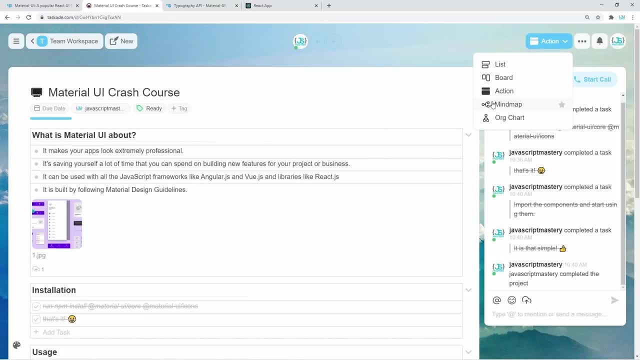 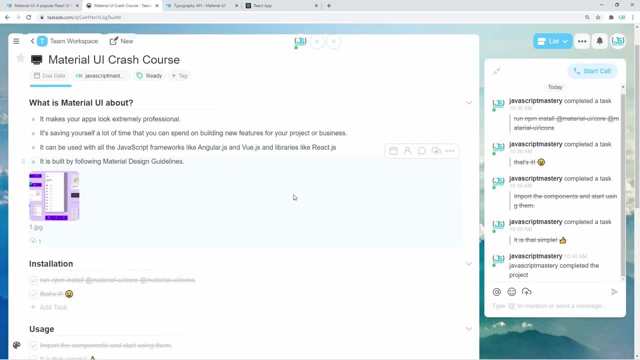 You can also create an action tab out of this or even a mind map. You can see how you can see that in different views. Once again, I cannot really recommend Taskade enough. I really want you to give it a try. You can have a lot of different task lists. 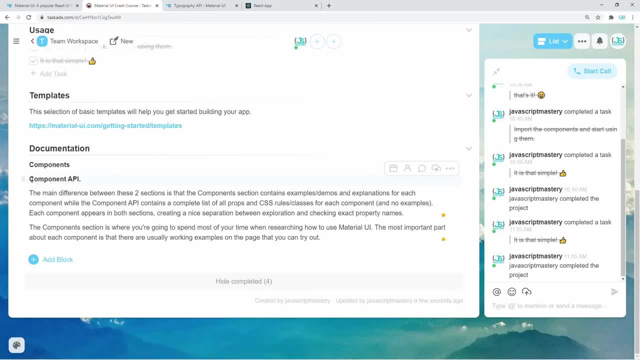 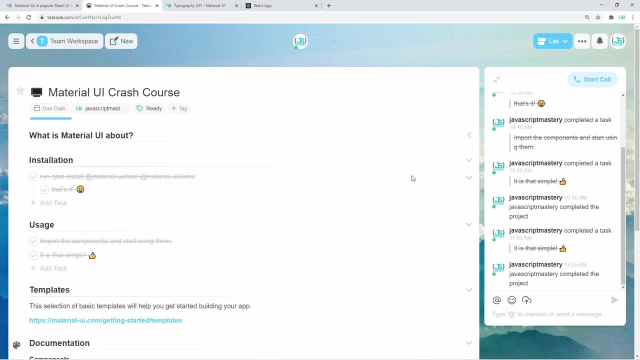 You can create different themes, add them together and, generally, it uses a really simple design where you can simply invent things that are grouped together. With that said, don't forget to shoot them an email to get the pro version completely for free. Let's continue with our Material UI project. 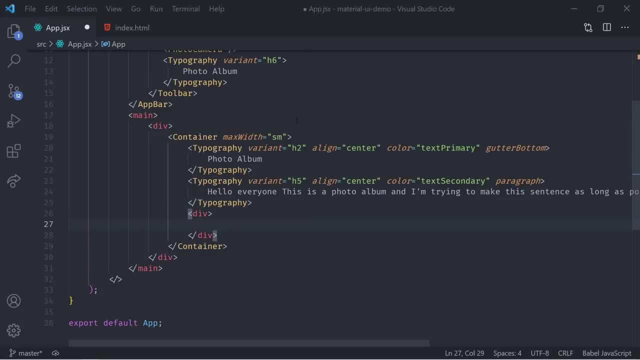 Right below this typography we're going to create another div. Inside of this div we'll want to position some content, and we do positioning and responsive design in Material UI using the grid component. So inside of here we're going to create a grid component, and they always come in pairs. 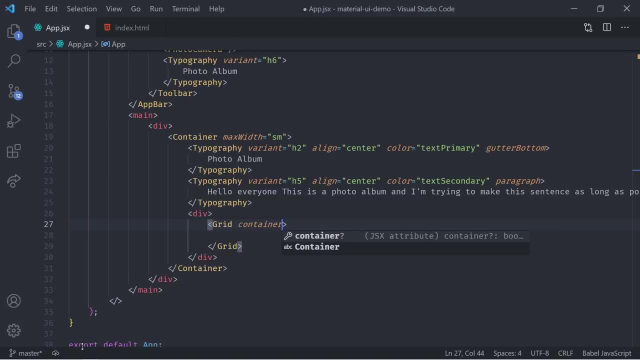 First you have a grid that is of a type container, and then in there you can provide some spacing between the element. So let's do spacing is equal to two, And then, in this case, we'll want to use the flex justify to simply center. 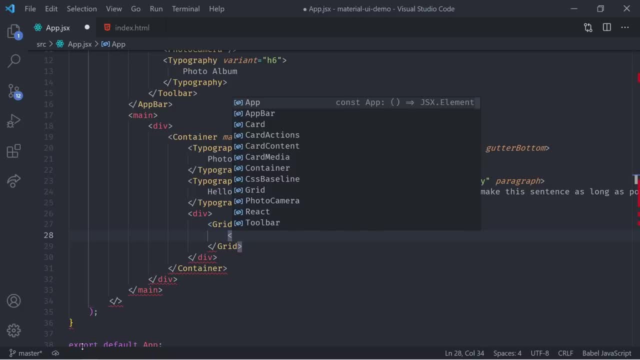 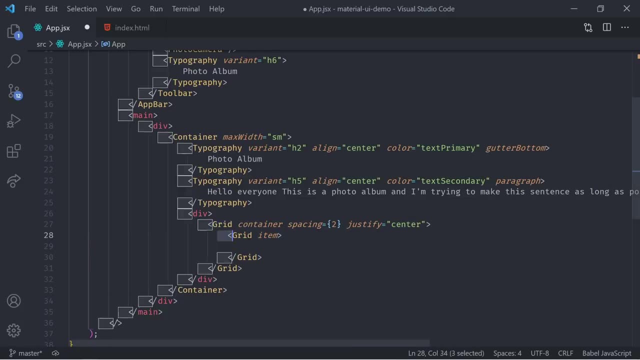 Now, inside of there, we're going to have the second pair and that is going to be the grid of type item. So you have a grid container that wraps grid items. Inside of this grid item we're going to have a button. 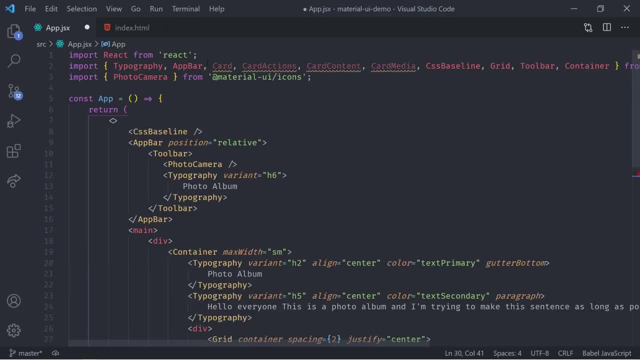 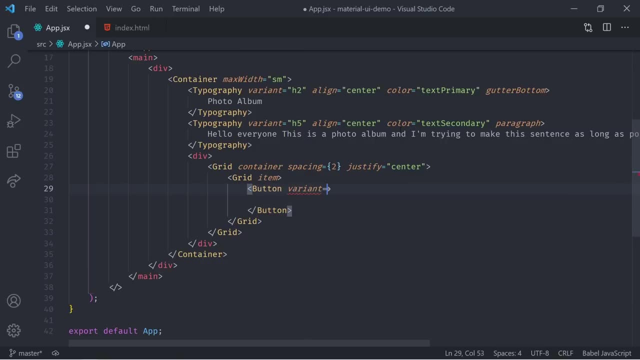 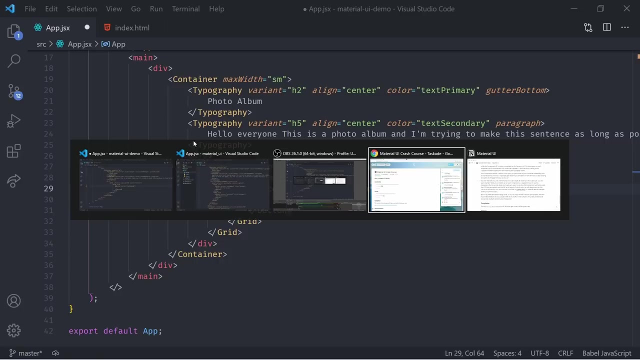 Okay, and I think I forgot to import it at the top, So we'll add the import right in here. This button is going to have a variant of contained, which simply means that it's all going to be colored. Contained simply is a style of the button. we can go to the Material UI documentation. 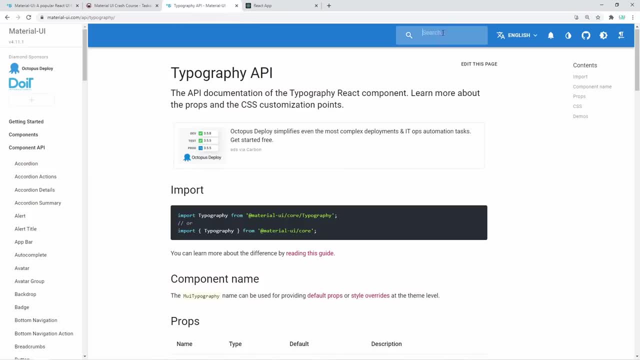 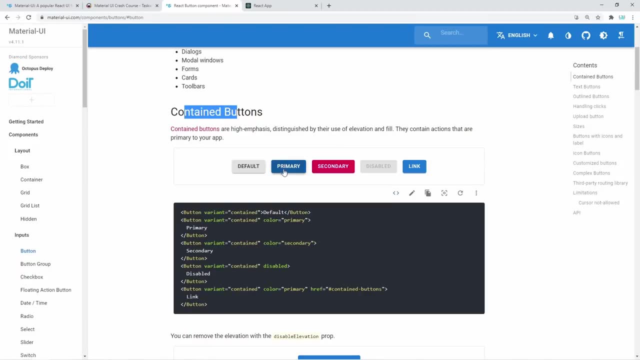 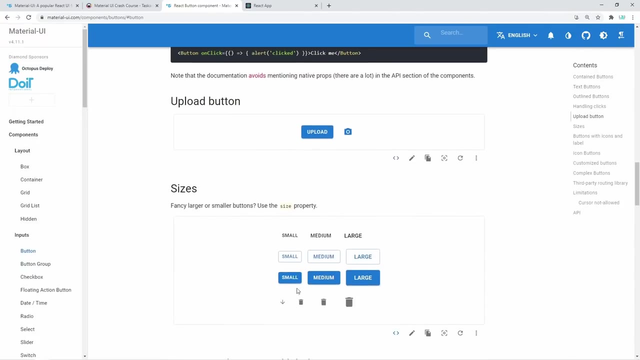 and check that out. So if we go right in here and if we search for the button in here, you can see that we have different styles. we have contained buttons which look like this. we also have text buttons, We have the outline buttons and you have a lot of different styles, sizes and so on. 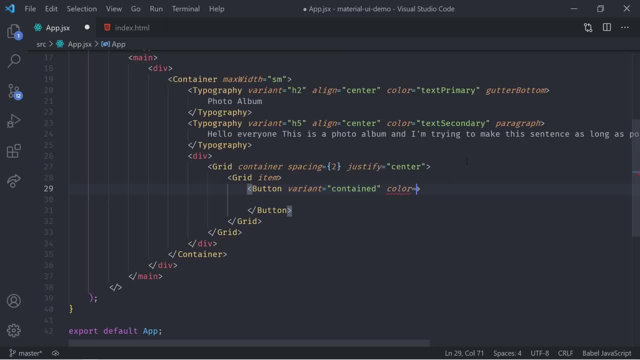 In this case, we'll simply use a contained button that is going to have a color of primary Inside of there. you simply want to say something. In this case, since we're working on a photo album, let's say: see my photos. 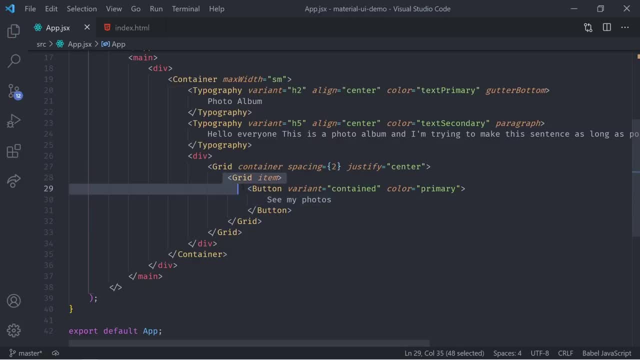 That is some sort of a call to action button. Below that, I'm going to copy this entire grid and simply paste it one more time. In this case, I'm going to put an outline button and the color is going to also say: 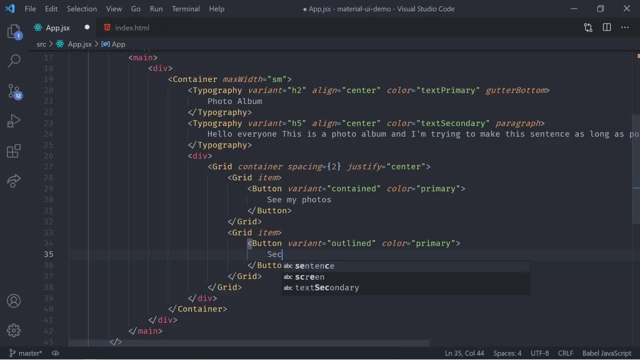 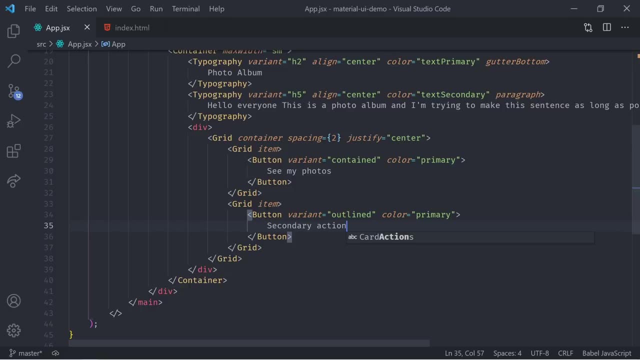 as primary. This would be some sort of a secondary action. So let's do secondary action. So now that we have these buttons in a grid, let's see how does it look like. If we go here, you can see that it looks really, really good. 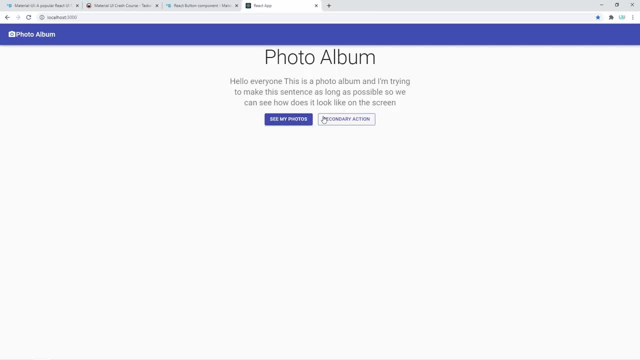 Again, keep in mind how much time would you have to spend to get this design just using plain CSS, And it still wouldn't look as good as this This looks right now. Also, something that is phenomenal about Material UI, which I really like, is that it is completely. 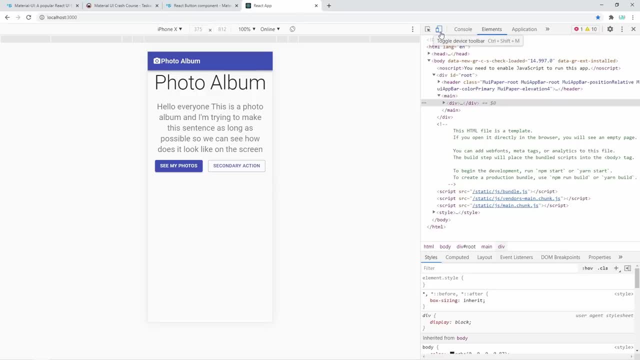 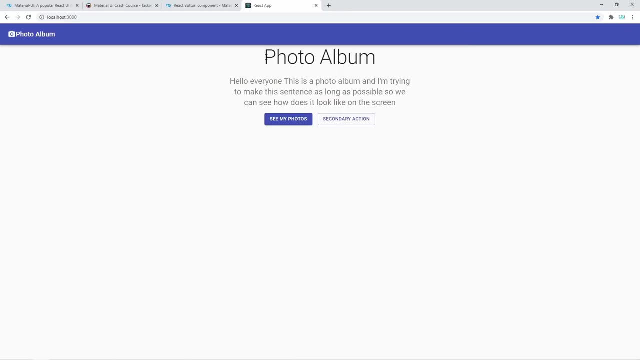 responsive. If you open the console and click right there on toggle device toolbar, you'll see that it is extremely responsive. The only thing that we have to do right now is just add some custom styling to add the margin top to this photo album and to center this on the page. 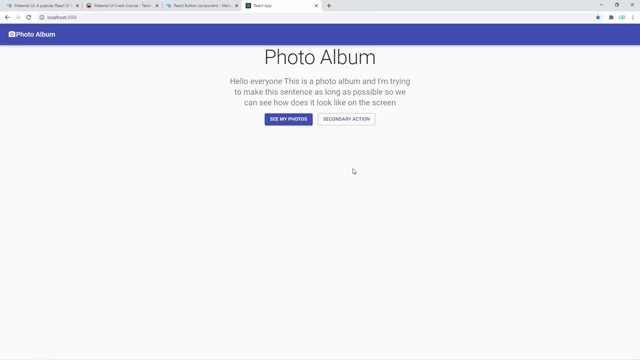 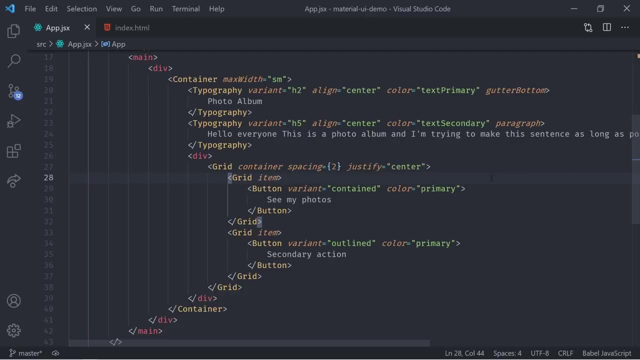 For that. we're going to go to our next lecture, which is learning about how to customize your material UI components. There are a lot of different ways in which you can style your material UI applications. There are a lot of different ways in which you can style your material UI applications. 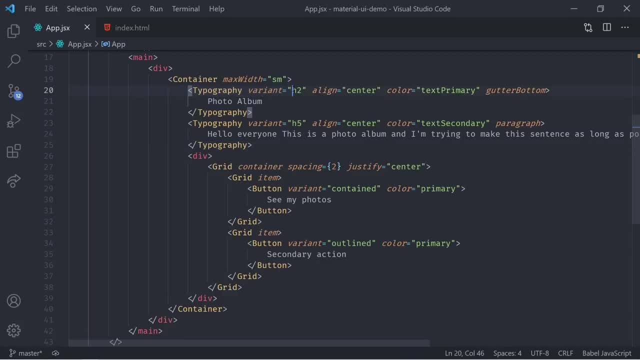 Of course, since we're working in React, the simplest way would be to use the inline styles. For example, if we want to provide a margin top to this container, you can simply say: style is equal to margin top, And then we can do something like 100 pixels. 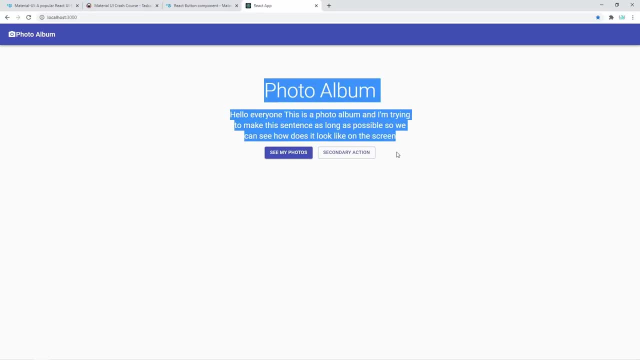 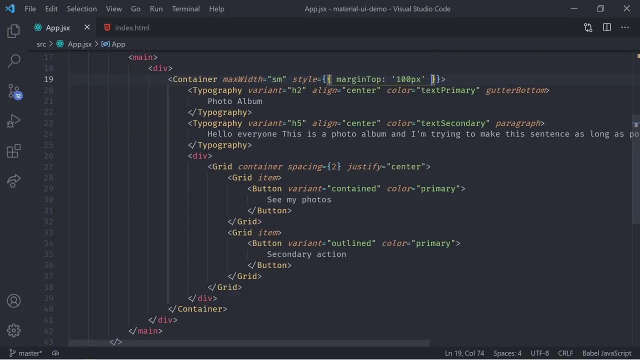 If we save that, let's see that in the browser. That already made it look so much better. But now imagine if you want to do some more complex styles. This wouldn't be ideal because you would clutter your view in the JSX and you would merge the 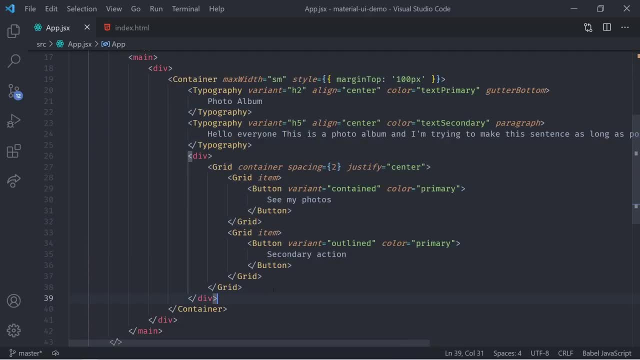 styling and the representation in one part. But now imagine that you want to do some more complex styles, like 3,, 4,, 10 different styles to each one of these components. That would clutter your view and your component would become really, really unreadable. 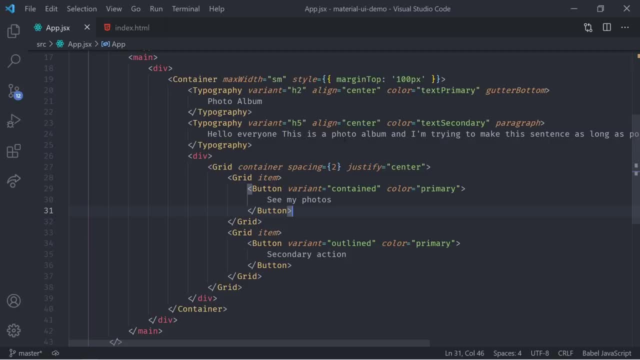 You don't want to put the styling right into your JSX. You want to have it separate. So let's explore different ways in which you can style your material UI applications in a better way. The best way is to use the material UI recommended styling. 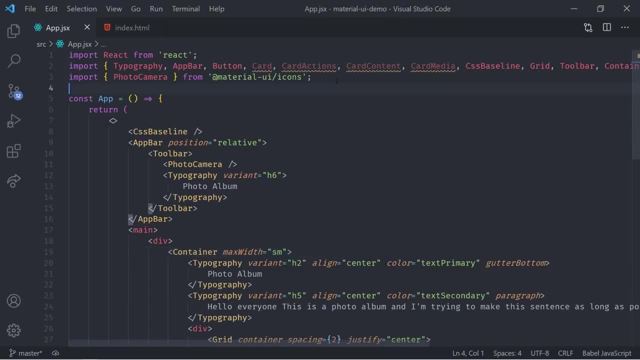 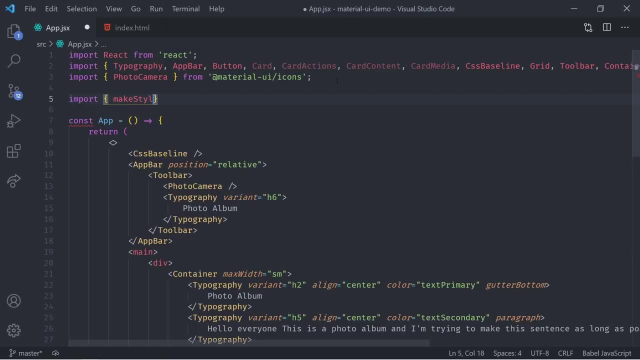 So let's explore how we can do that. First, we'll have to scroll up and you're going to have to import something called the material UI application. Let's do that. We're going to call it make styles. So import, make styles and that's going to be coming from at material UI forward slash. 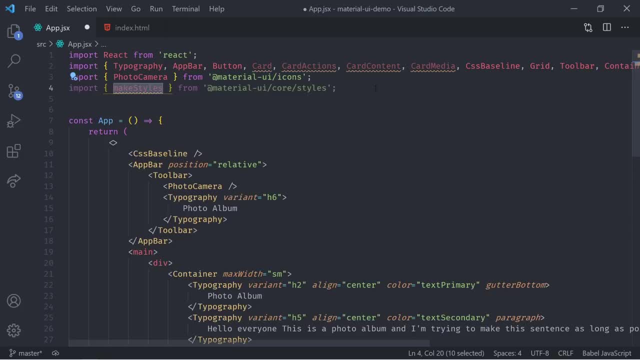 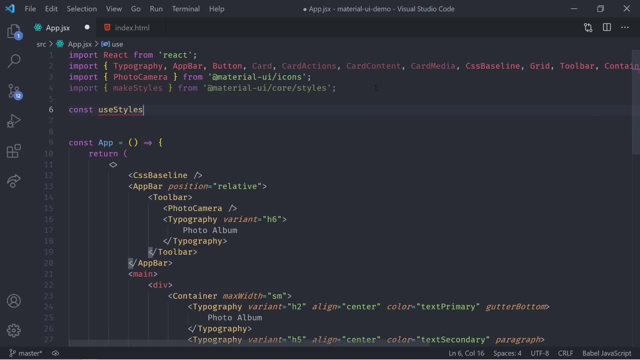 core forward slash styles. Now that you have these make styles, we're going to create a hook called use styles So you can say: const use styles is equal to make styles. Bear with me, I know that the syntax is a bit confusing. 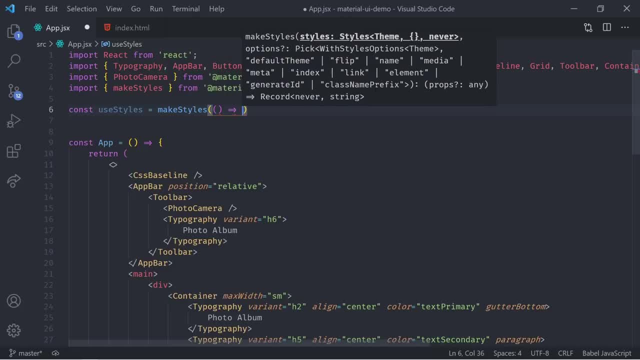 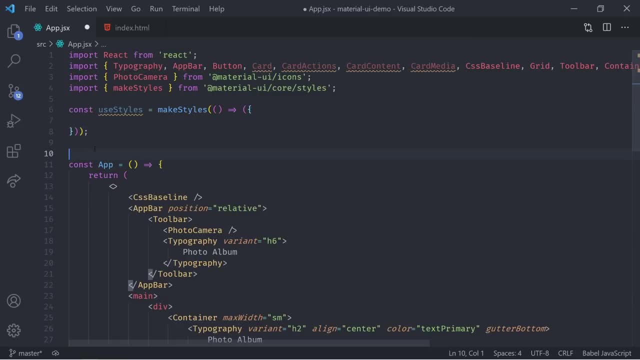 And then in there You have a callback function that returns an object. So this is the syntax. I know that it is a bit confusing, but let's go through it line by line, or rather word by word. We're creating a hook called use styles. 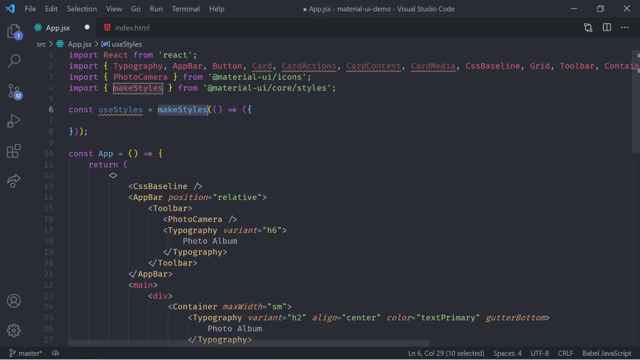 That is equal to to a function call called make styles. Inside of that function call we pass in a callback function that simply immediately returns an object which contains all the styles. Make sure to rewatch this a few times. I know it can be confusing. 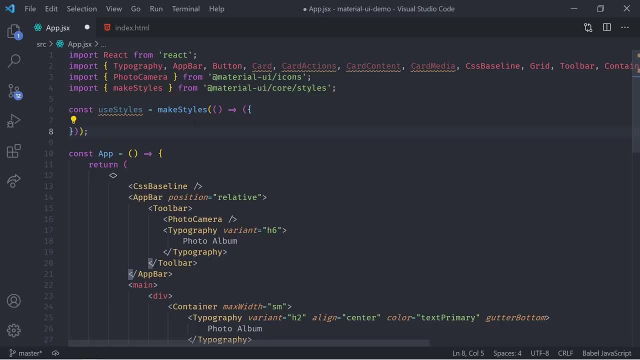 But once you get used to it, you're just start creating these styles really quickly. In here we also get access to the theme, which you can use to provide additional styling. Now that we have this hook, we have to create classes object out of it. 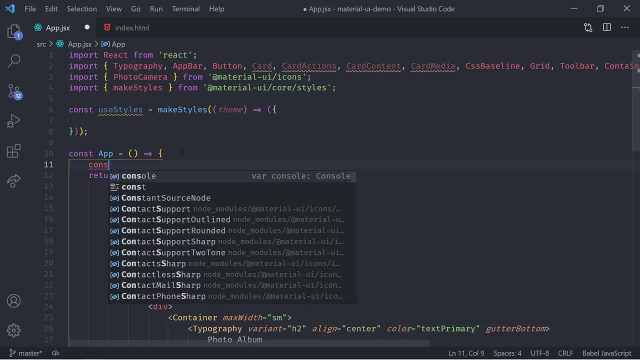 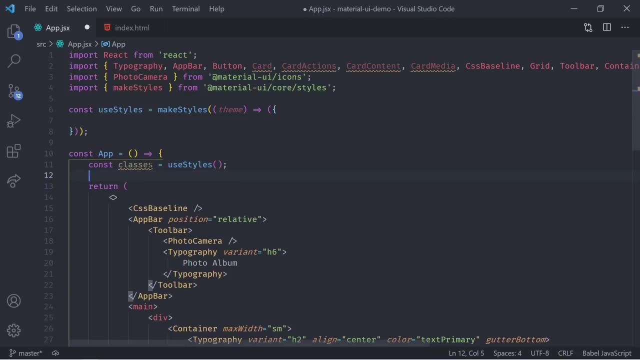 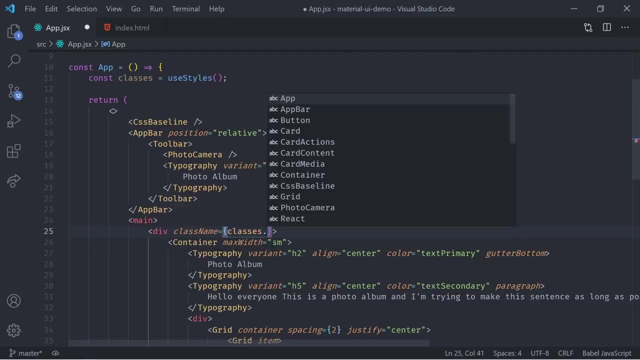 To do that you need to go inside of your component and say const classes is equal to use styles, and then you call it as a function. To provide a class to an element, you simply need to say class name is equal to classes dot and then you can think of a name. 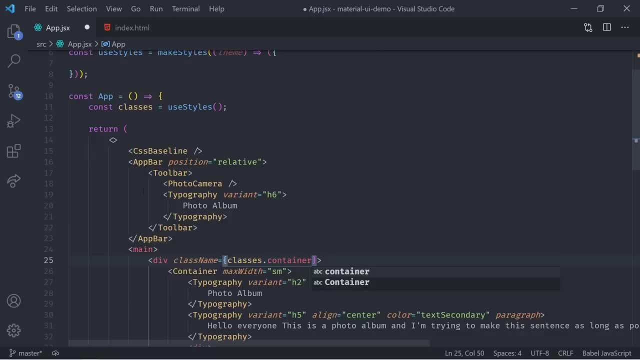 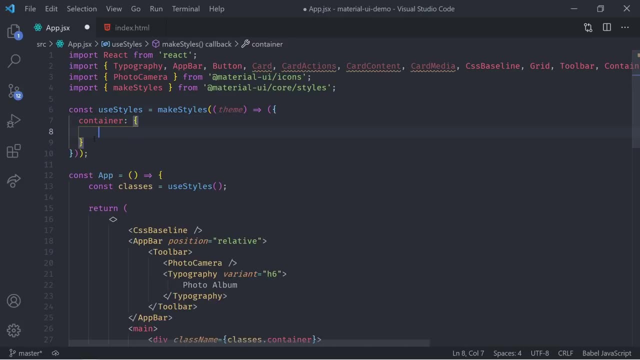 In this case, let's go for a container. Now in this object you need to create a new object called container And in here you provide the styles. I know it's a bit unorthodox to people who were just writing styles in the CSS. 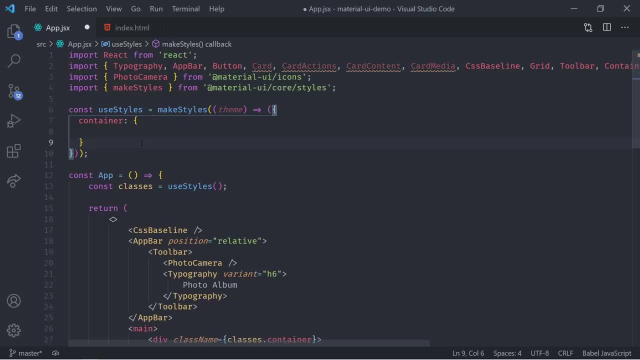 But material UI uses something known CSS in JS, and this is how we write styles. I know it's not perfect, but if you get used to it, material UI is going to really allow you to do a lot of things with dynamic styling. So what are we going to do for our container? 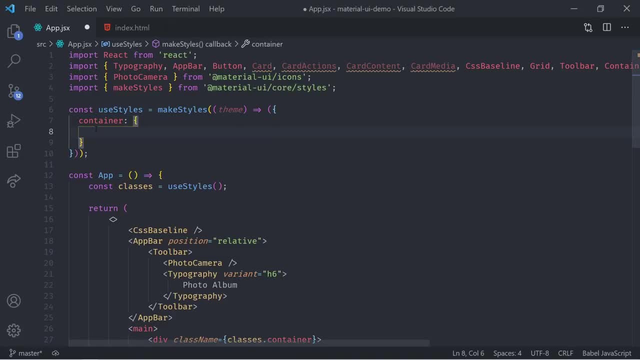 Well, for example, let's try adding a background color. You can simply say background color and that is going to be equal to any color, But in this case we're going to use material You guys built in background color, and how can we do that? 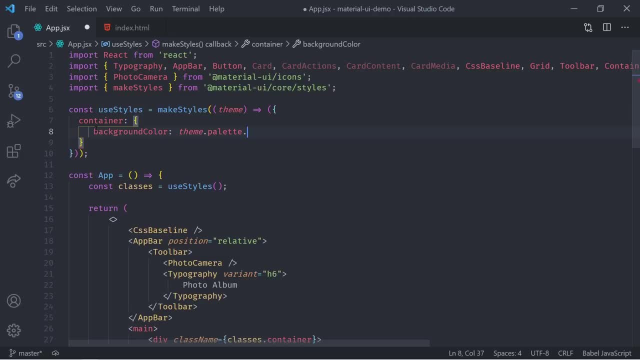 You can say: theme dot palette dot background dot paper. This is going to give you a lightish background color. Also, let's give it some padding. You can say padding is equal to theme dot spacing and then in here you can provide different spacing as a function. 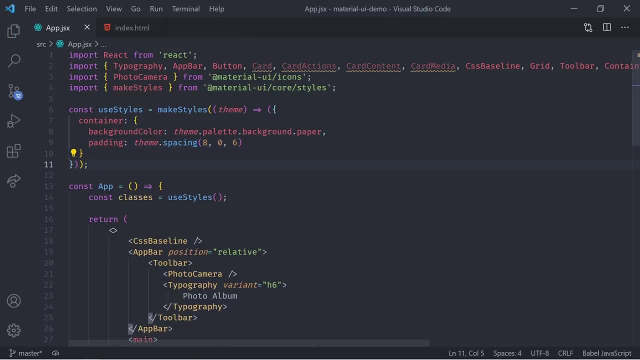 We're going to do 806.. I know this might be a bit confusing, but you don't have to use this. You can just use. padding is equal to something like, you know, 20 pixels. I just wanted to show you that you have this theme object which you can explore on material. 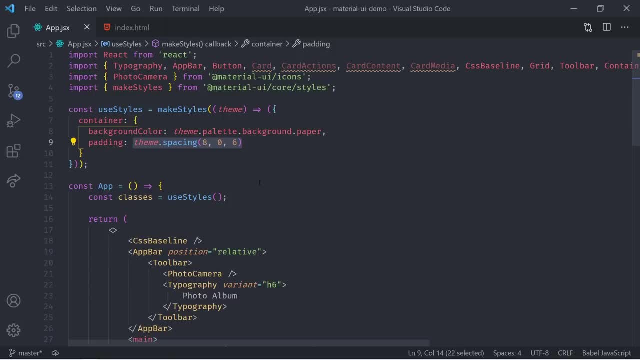 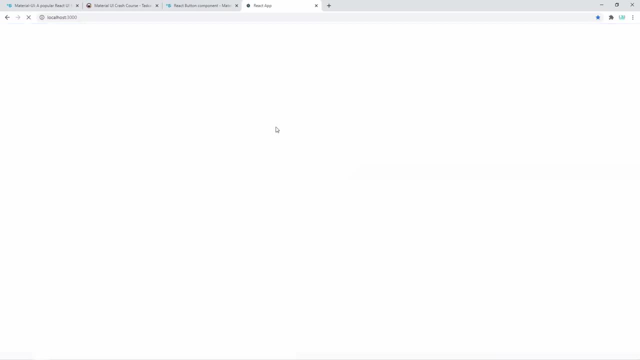 UI's website, and it provides you certain padding measures that you can use all across your application. With that said, let's save this and see if it worked. If we inspect this page, as you can see, it added the padding to this main div and then 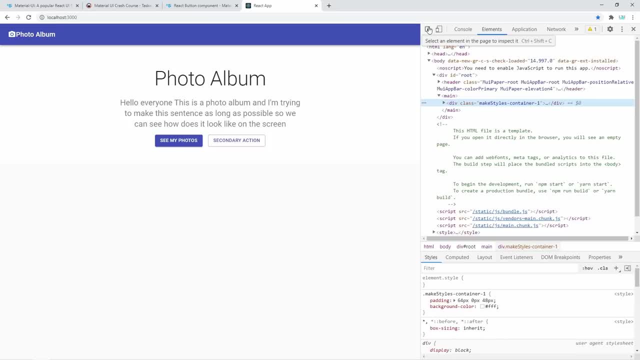 also, it added a background color of white and, because of our CSS baseline, everything else has this grayish color. I'm not sure if you can see it on the screen, but it is there. There is a difference between those two colors. It's really subtle, but it is there. 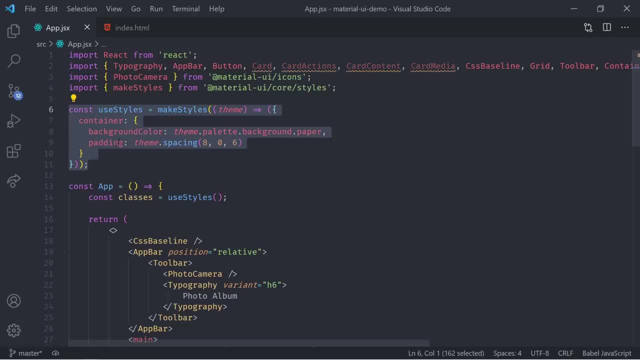 With that said, as we keep adding more styles, we're going to still clutter our view from our app JSX. We're going to have the imports and then hundreds of lines of styling and then the JSX. So what I prefer to do is create a new file just for the styles. 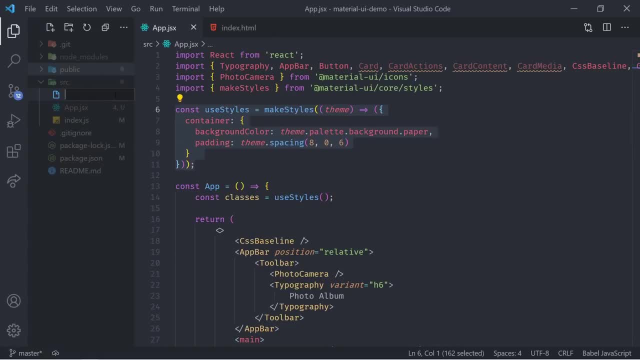 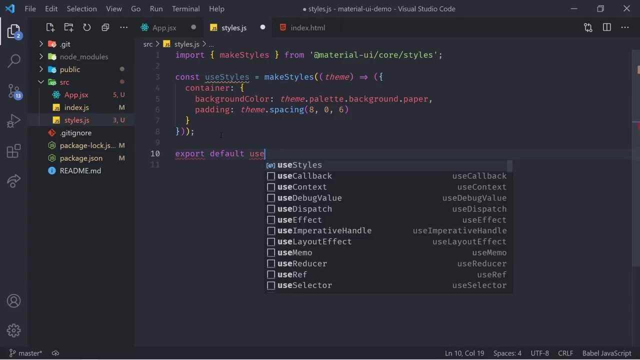 And you can do that easily Inside of the SRC. I'm going to create a stylesjs file Inside of here. we're going to import everything we mentioned about the styles. Okay, and now the last thing that you have to do is just say: export default use styles. 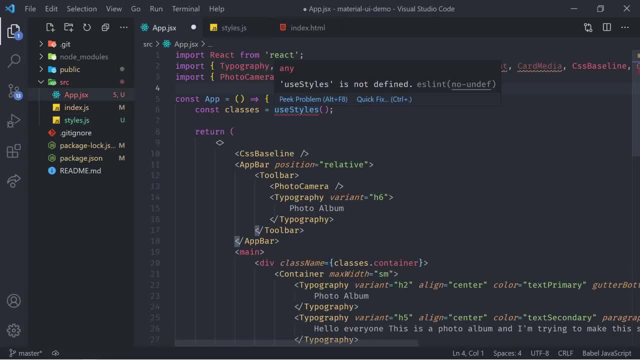 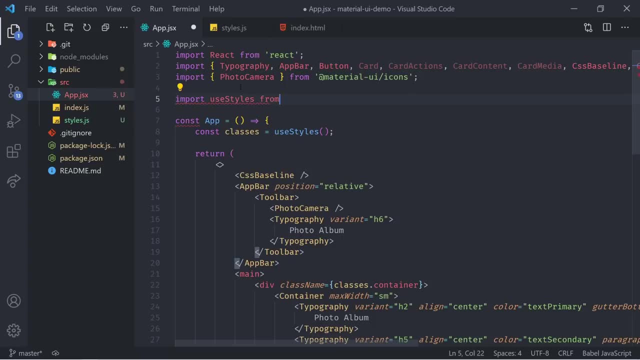 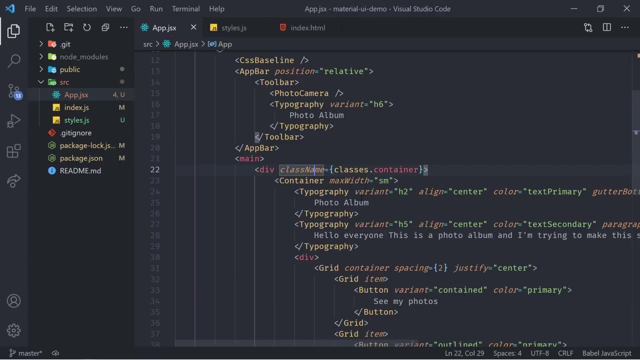 So now these styles are being exported and you can see we're missing them right here. but we can simply import them by saying: import, use styles from JSX And that's going to be dot slash styles- Great. So now we have only one line. we're not cluttering our view with any inline styles, we're simply 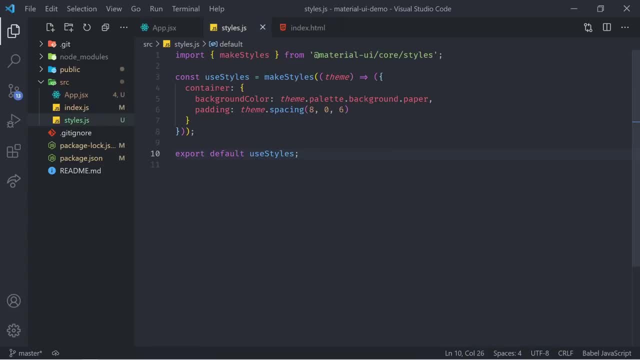 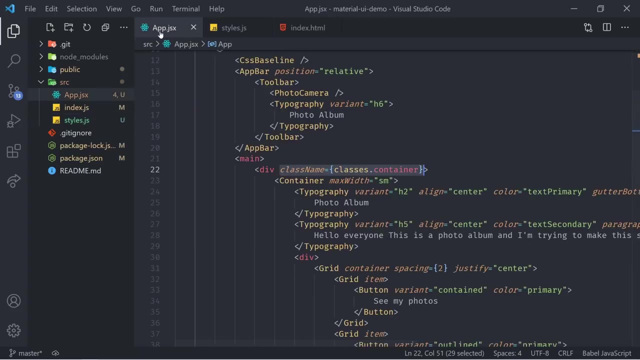 going to use the class names that we're going to add the styles for right in here, And I know it might be confusing, but you're going to get used to it if you start using it more and more. At first I hated this CSS in JS type of styling, but later on I grew used to it. 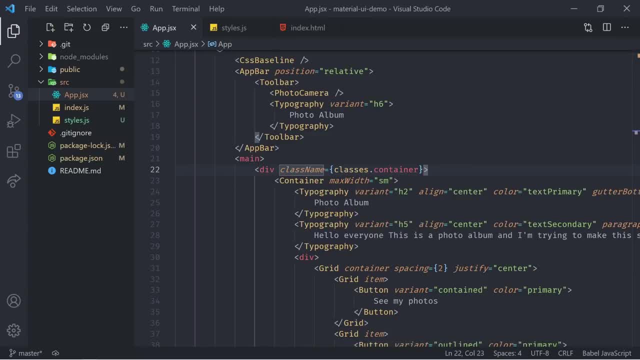 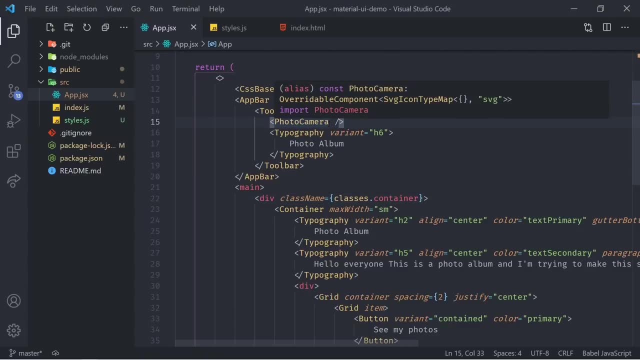 So now let's continue. Let's continue adding some styles that we missed, maybe, at the start of our application. In this case we also want to add the classes for our icon. So in here I'm going to say: class name is equal to classes dot icon. 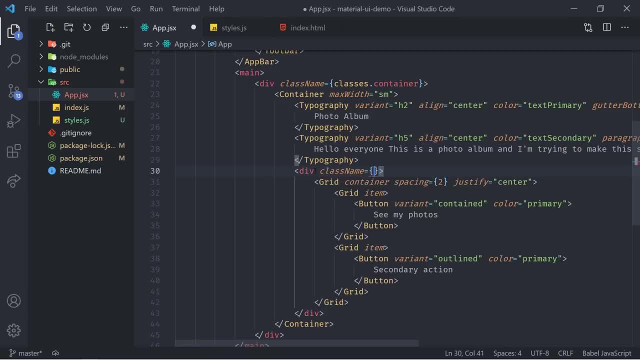 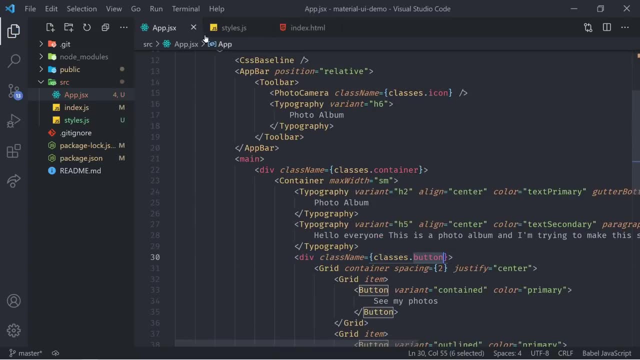 Also in this div for the buttons I want to say: class name is equal to classes dot buttons. So now we know that we have to add the styles for the icon and the buttons, So I'm going to open this on the side And then in here. 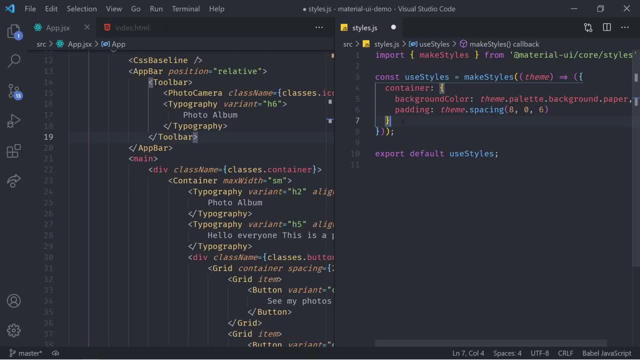 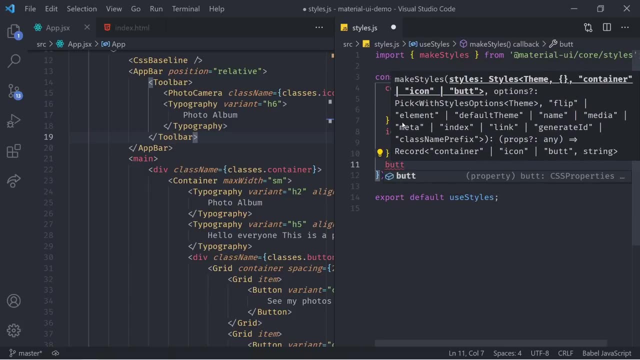 I'm going to add those styles. You can simply add new objects. So just below the container, I'm going to say icon And I'm going to also open the new object for the buttons. Okay, so what styling do we want to add? 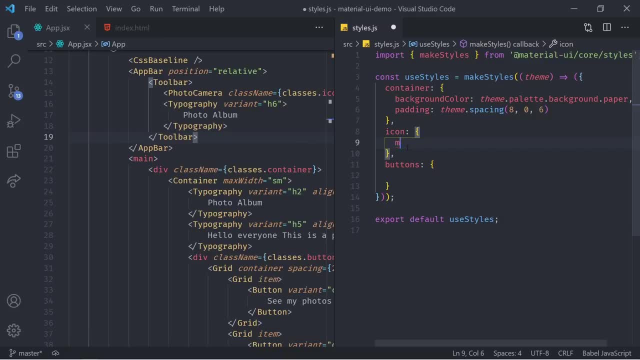 Well, for the icon, we want to give it some margin right. So I'm going to say margin right And you could do something like theme dot spacing, and then you can say two. But you don't really have to. you can simply say something like: let's do 20 pixels. 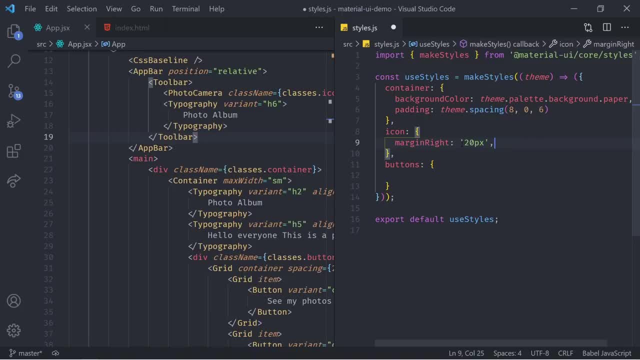 And keep in mind, all the styles in CSS and JS need to be wrapped in strings. Okay, and then for our buttons, we're going to do margin top And let's do something like: let's do 40 pixels, Great. 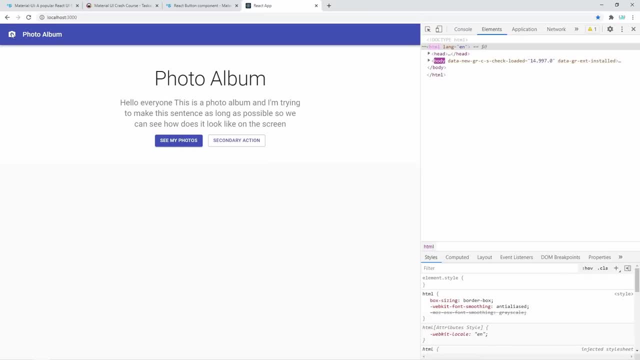 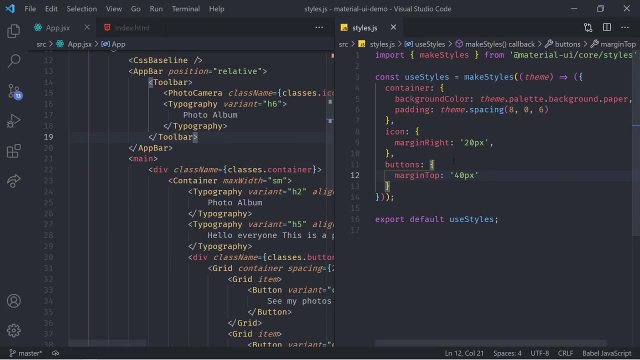 Now that we have that, let's see how does it look like? Great. So we added some differentiation on the top left side. we have some margin there and we added the margin top On our buttons. of course, we misspelled it here. 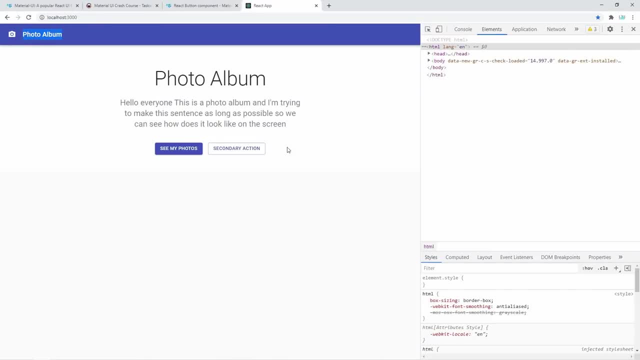 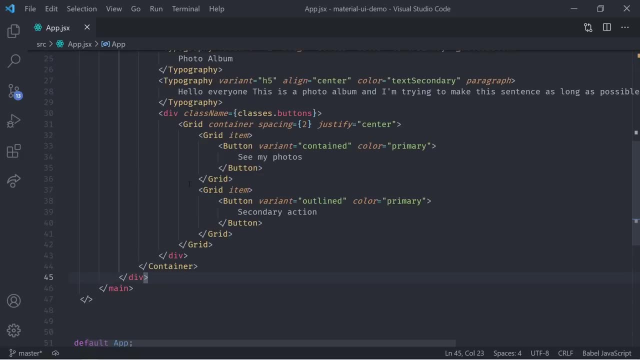 So if we fix it, you can see that looks so much better now. Now that we covered the styling, let's keep moving forwards with adding new components to our application. Next, below our div for the container, right in here, we're going to create another container. 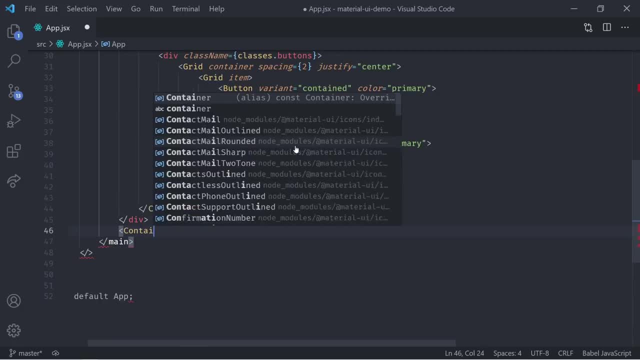 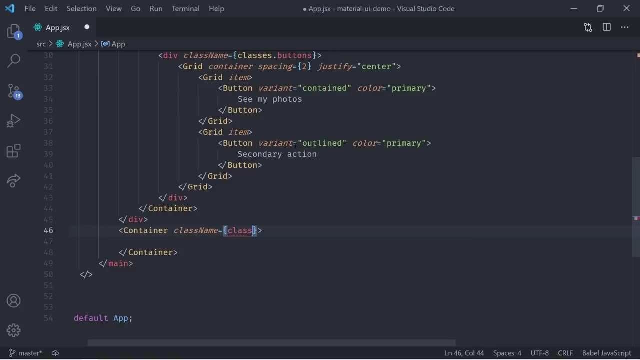 This one is going to be for our cards, So let's go ahead and create a new container. This container is going to have a class. It's going to have a class name of classescardgrid. It's also going to have a max width of MD, which stands for medium. 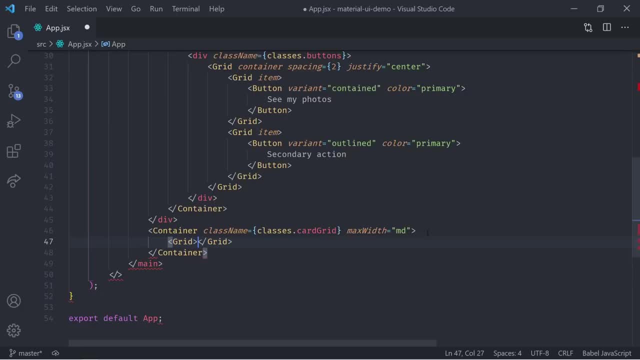 Inside of there, we're going to use a grid. We already learned what grid is. It is simply for responsive design and for positioning some things on the page. We also learned that we first need to have a grid container with some spacing. Let's do four this time. 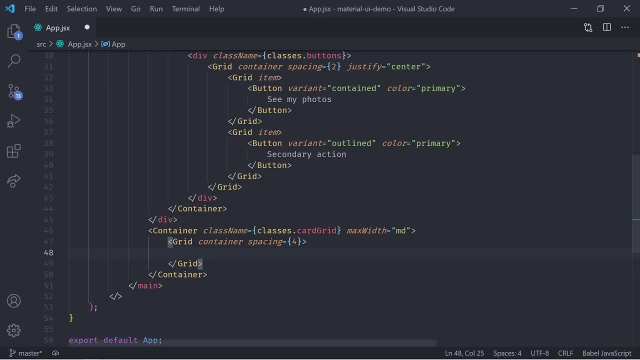 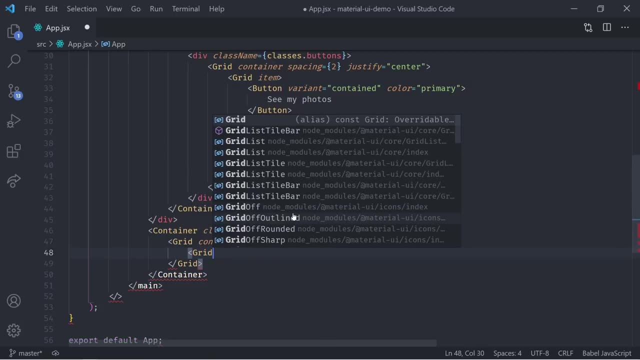 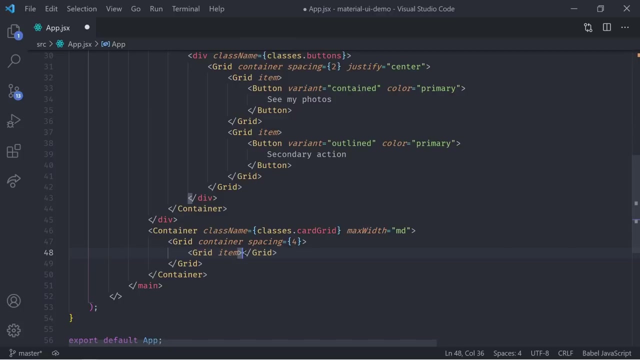 And then inside of there We have to have a lot of grid items. In this case, our grid item is going to be a card, So let's do that grid. It's going to have the property of item. Inside of that grid we're going to have a card element. 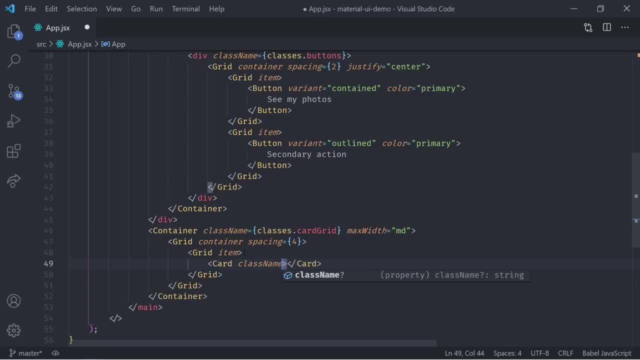 That card is going to have a class name of classescard. We're not adding the styling yet. We're going to add it as soon as we're done with this part. We're going to have a card media which is used for the image. 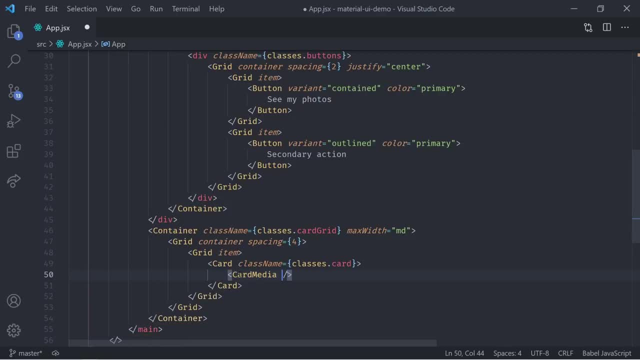 That card media is going to be a self-closing element, So we don't have to have any opening and closing elements. It's going to have a class name which is going to be equal to classescardmedia. It's also going to have an image property. 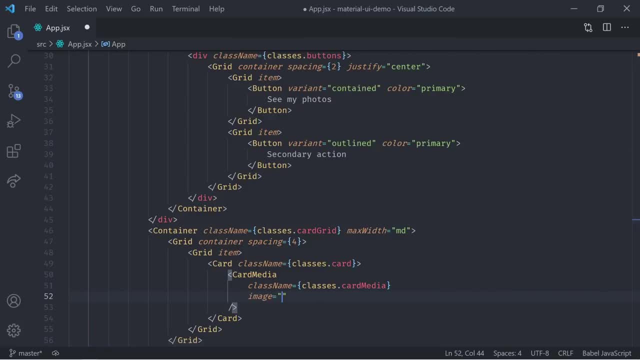 And that image is simply going to be an image from the web. In this case, we can use the image from Unsplash- That's going to be https//sourceunsplashcom, And they have this nice library called random, So you're going to get a new random image every time that you visit the page. 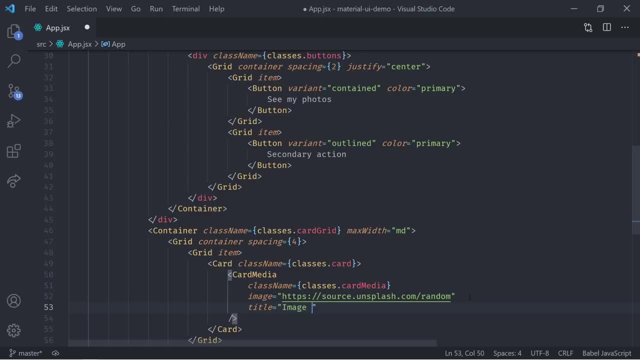 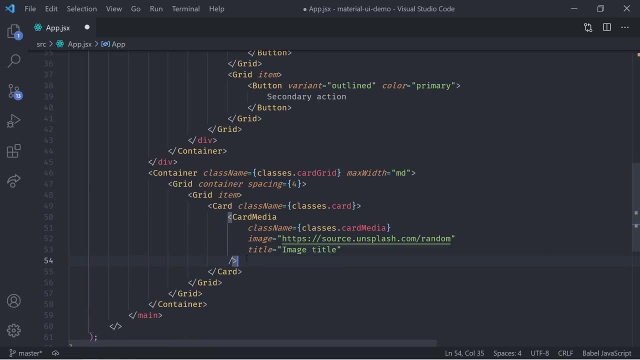 And finally, we can have a title. This is going to be something like image title. We don't have to focus on it right now. Each card also has a card content. So just below the card media we're going to have card content. 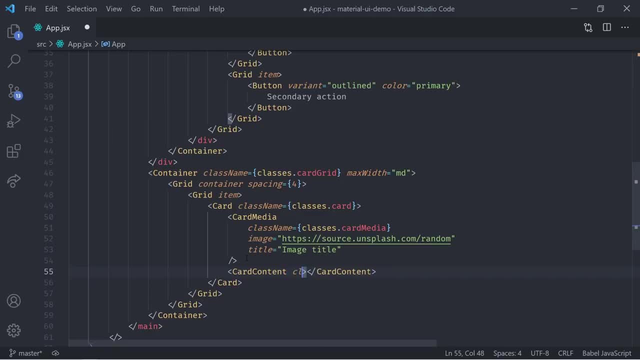 That card content is going to have a class name of classescardcontent And then inside of there you can provide all the content for your card. Primarily that is going to be a typography. This typography is going to have a gutter bottom and a variant of age five. 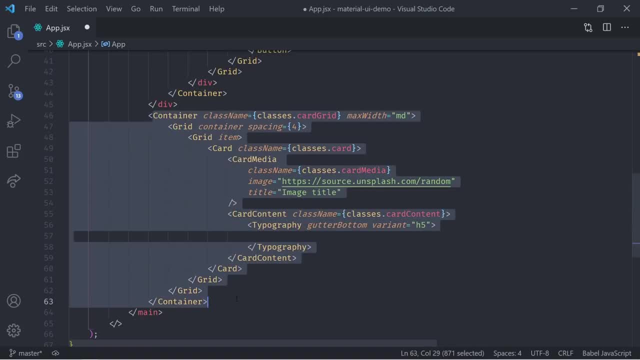 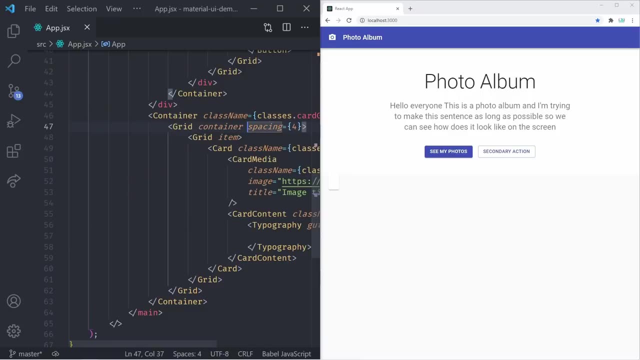 And now that I'm thinking about it, it would be great. Okay, So let's start with the code, While at the same time, we're looking at the changes that we're making. So I'm going to put the window side by side. 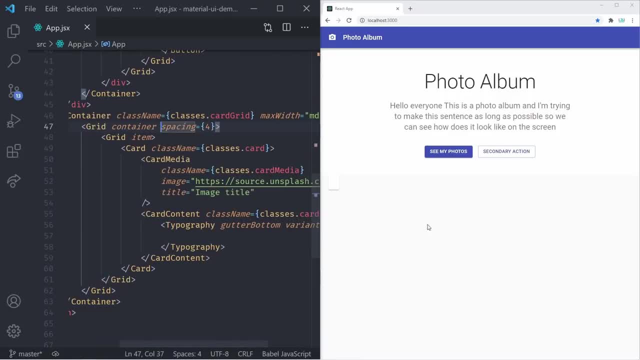 There we go. Our windows are now side by side, So you can see in real time what we're creating right in here Right now. you can see it is basically nothing. It is an empty div. It's really invisible right there, Okay. 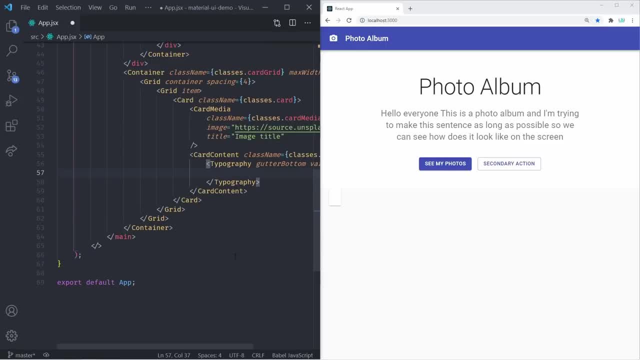 Let's keep adding more stuff so that you can see what we are creating. Furthermore, our typography is going to have a heading Okay, And then we're going to have one more typography below this one. This typography is simply going to say: this is a media card. 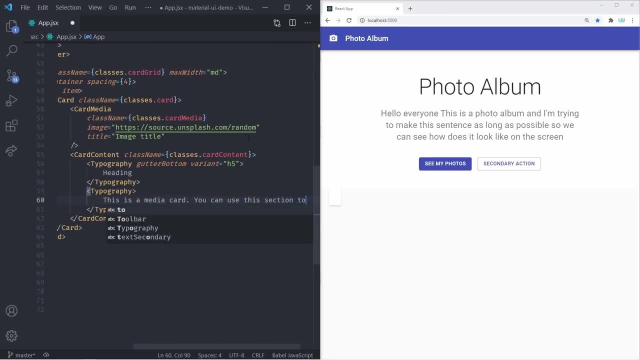 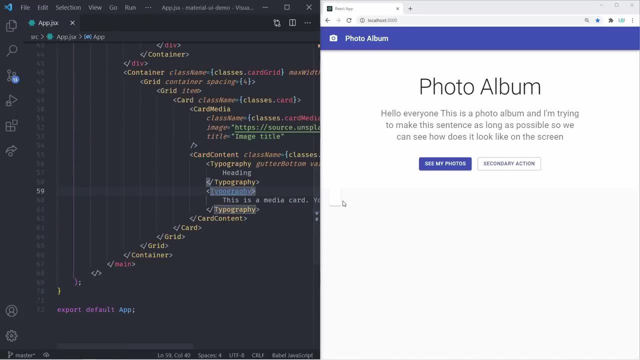 You can use this section to describe the content. Great. So now we have this typography, Let's save it. And, as you can see on the right side, this is already starting to look like a card that we want to use. Finally, 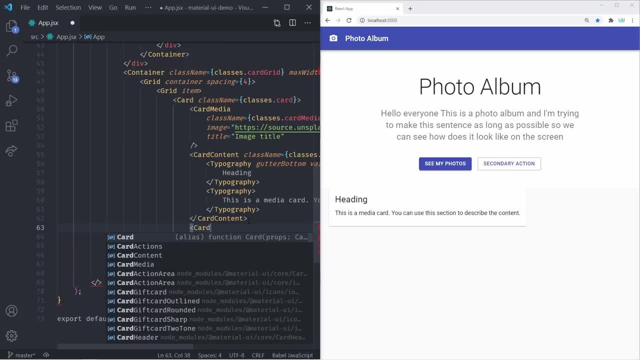 The card content. we're also going to have card actions. Card actions is a bottom part of the card where you want to put some buttons in, So let's do just that. We'll use two buttons. The first button is going to have the size of small and it is also going to have a color. 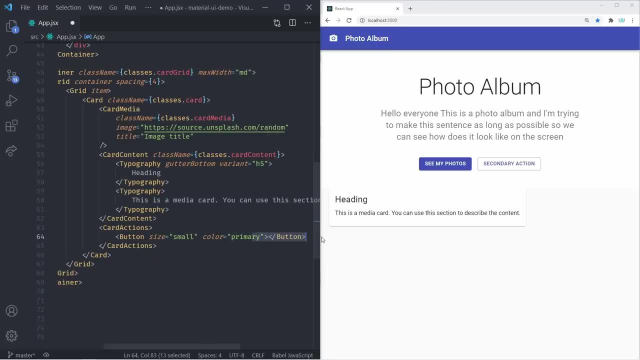 of primary. First, one can say something like view. Let's say that we have a lot of photos, We want to view the first one, We can replicate this line And the second one is simply going to say edit. If we save this, you can see we have this nice looking two buttons. 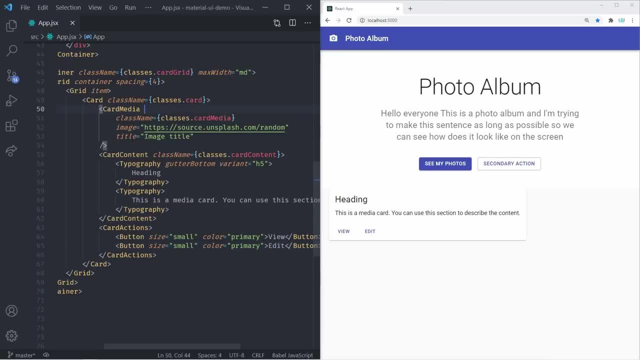 Great. Now what you might be wondering is: where is our image? Well, the thing with images is you have to give it a height, Otherwise it's not going to know how high it is. So what we have to do is we have to start adding some classes. 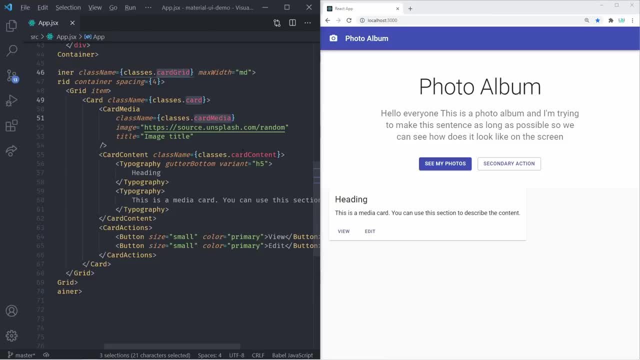 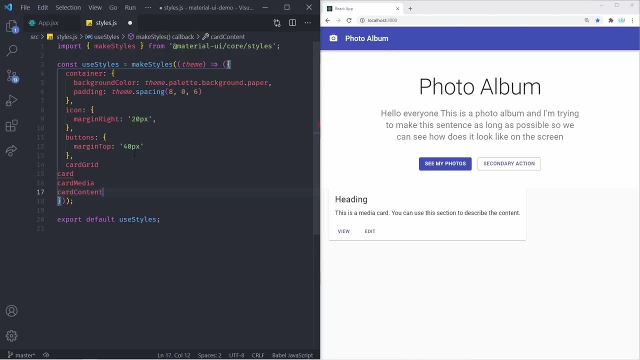 Remember, we added the card grid, the card card media and card content. So now we have to go to our styles and we have to provide a specific styling for each one of these classes. So let's do just that. Okay, I'm going to use some shortcuts magic to create this. 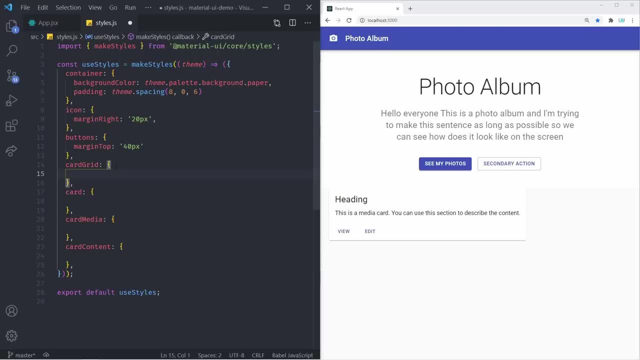 If you want a video about Visual Studio Code shortcuts, just let me know. Like this video: comment down below. With that said, let's start with our card grid. Our card grid is going to have a padding top, Or we can just do padding, and that's going to be equal to: let's do, 20 pixels on top and 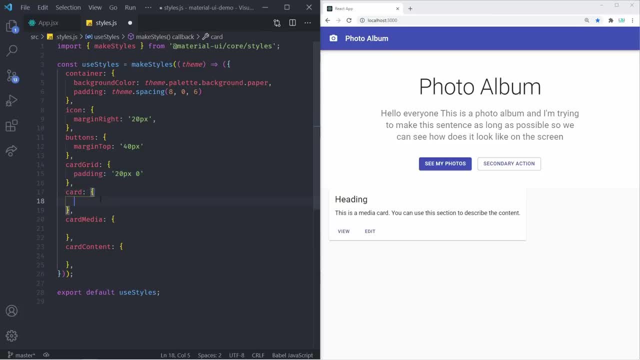 bottom and zero on left and right. Our card is going to have a height of 100%. It's going to have a display of flex as well as flex. direction is going to be column. Again, if you're writing code in CSS and JS, left side needs to be in camel case. 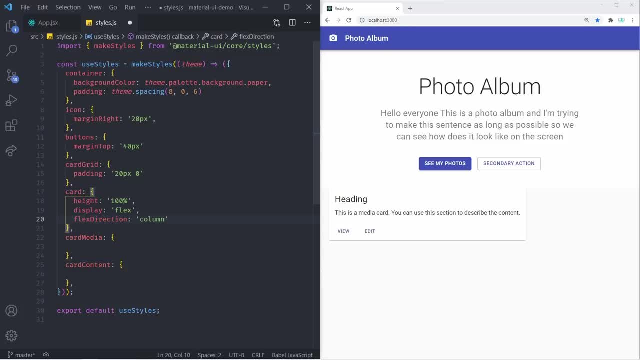 You cannot have something like flex direction like this: Okay, It has to be camel case, And then the right side has to be in a string. Finally, we have the card media. Card media is going to have the padding top of something like 56.25%. 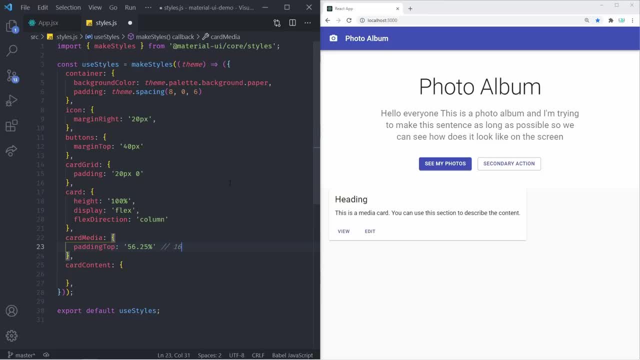 This is not a magic number. With this, you're simply getting an aspect ratio of 16 by 9, which is how you're used to seeing the images in this image ratio. Finally, the card content is going to have The flex grow, which means it's going to expand fully to one. 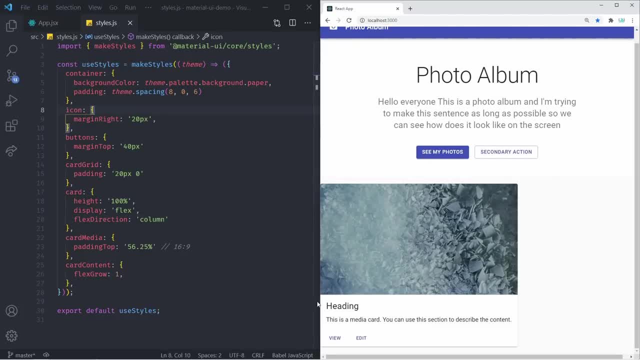 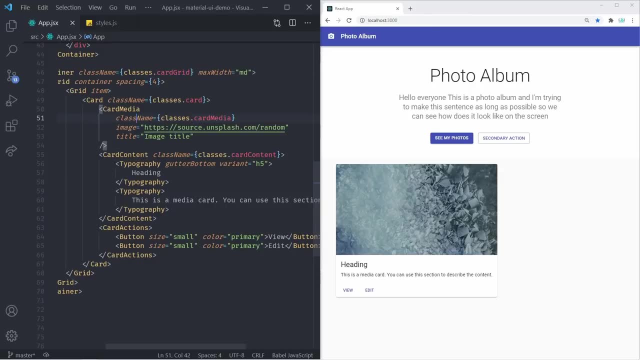 These are our styles And if we save it, you can see on the right side we have this nice looking huge card that has the image right now: Great. So this is going to be our card, but let's say that you want to have 10 or 20 different. 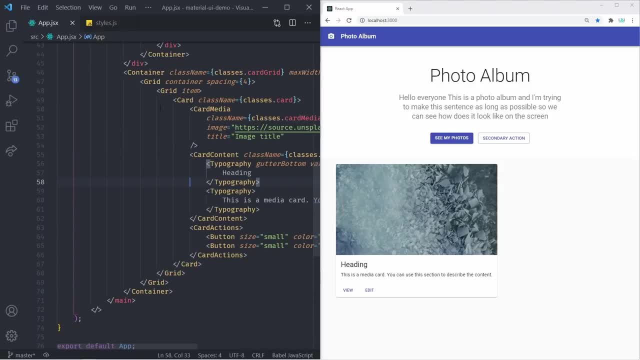 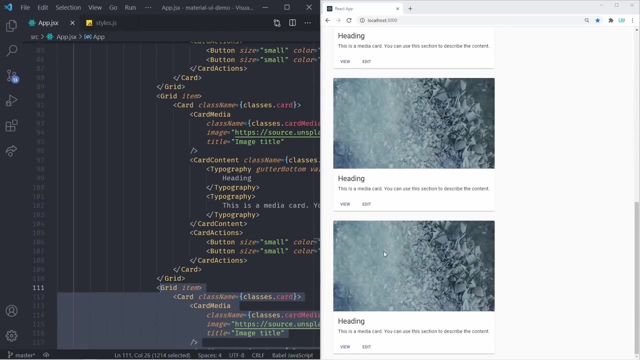 cards. What would you have to do? Well, one would assume that you can simply take the grid item, which is basically the actual card, and we can replicate it a few times down below, like this: Let's save it And, as you can see, we have this grid items going one below another. 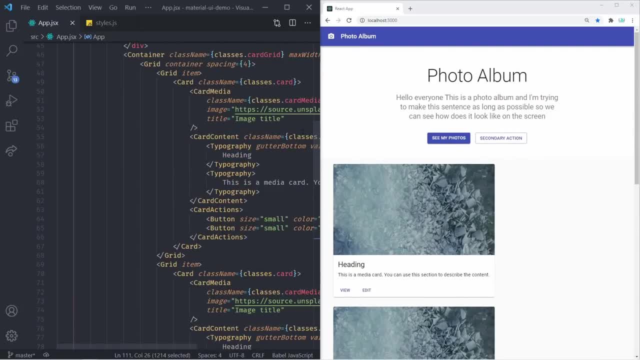 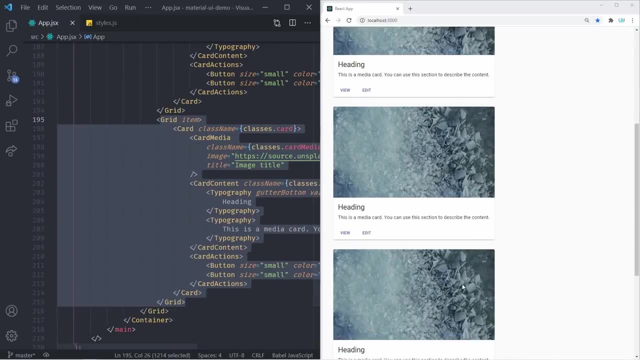 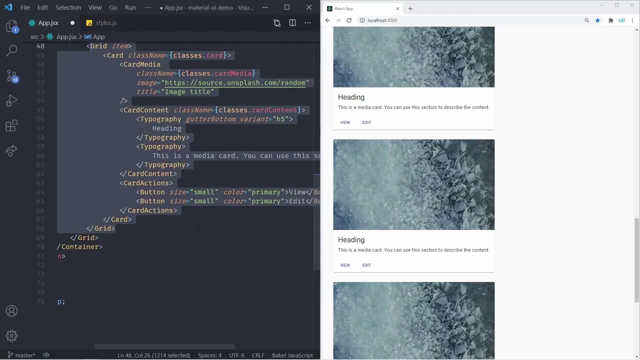 But again, take a look for something simple as this website. You just brought your code to have almost 150 lines, And if you just added like 10 more of these, your code would have more than 200 lines. So that's not going to be the solution that we're going to go for. 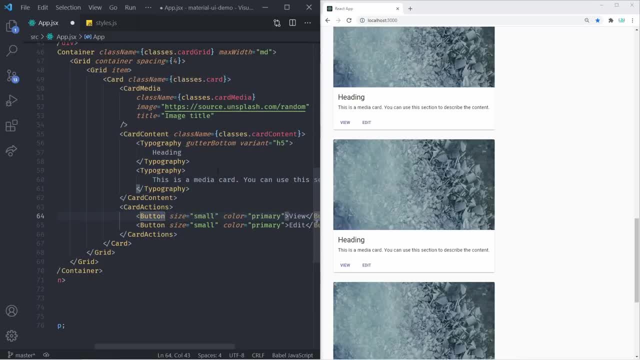 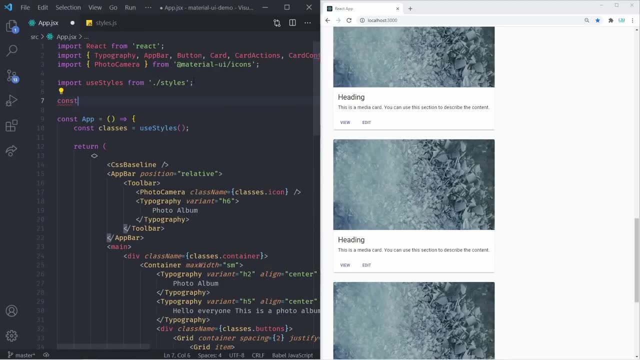 Our solution is going to be mapping over our items. So how can we do that? Well, first of all, let's create an array of different cards. So in here I'm going to say: const cards is equal to, and let's do 1,, 2,, 3,, 4,, 5,, 6,, 7,. 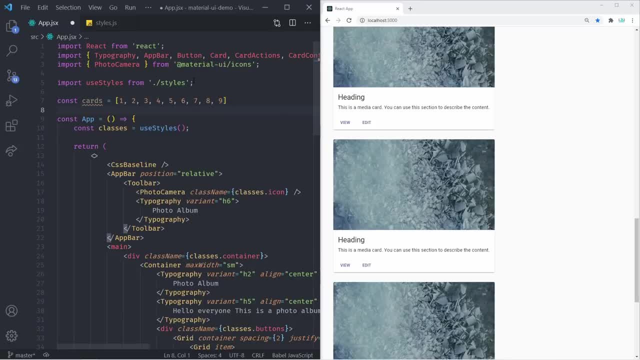 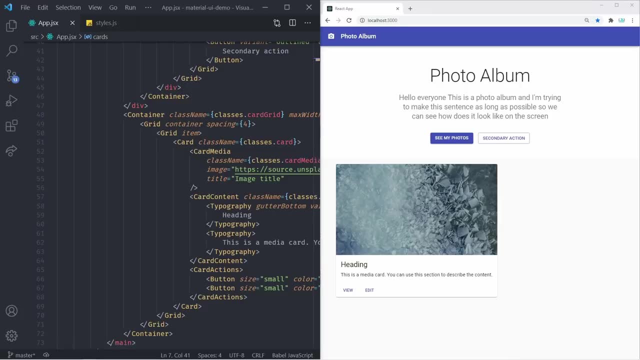 8,, 9.. We're going to have nine different images. Great. Now we can loop over those images to show the cards. We're going to loop over them right inside of our grid container. So right inside of here You can open a JSX logic block and you can say cardsmap. 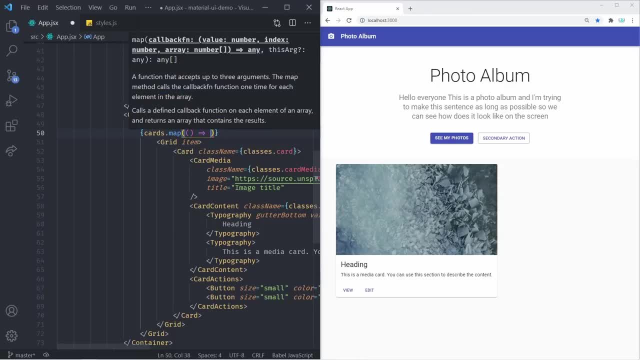 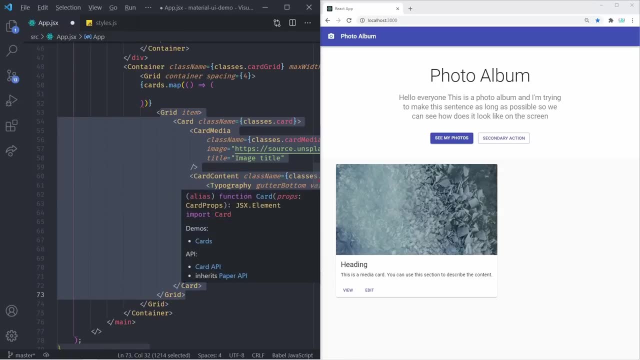 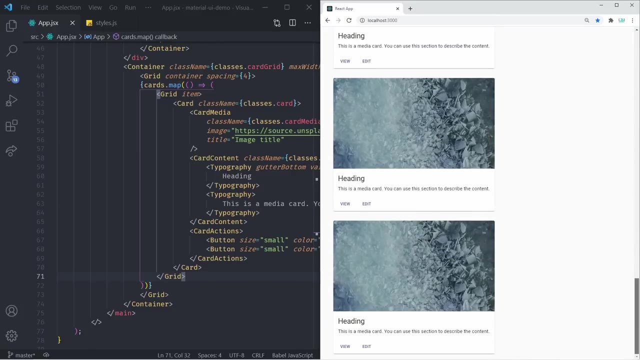 Of course, you need to open a callback function and we're going to have an instant return. Keep in mind, this is a parenthesis, not a curly brace. And now you can simply put this entire grid card inside of our map And just like that. as you can see, we have nine different cards while still remaining. 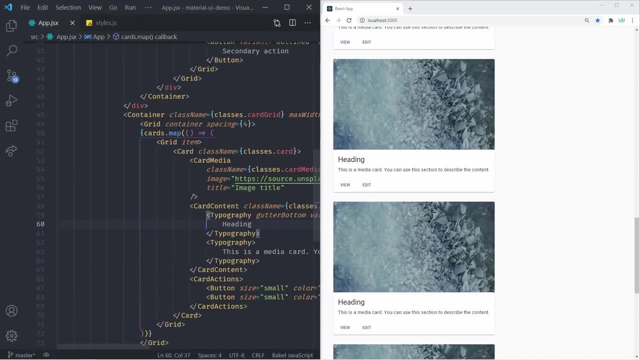 at 78 lines of code. That is great. Whenever you're mapping over something, you need to get the actual card and then you have to provide a key. In this case, the key is simply going to be the card. But again, this is not ideal because we are on a desktop. 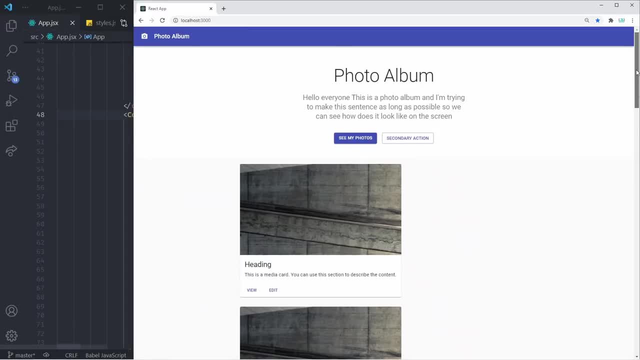 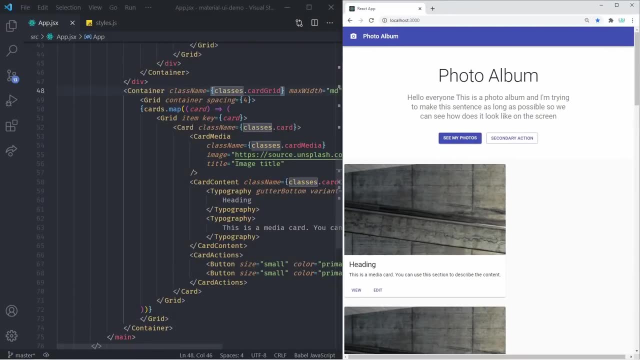 And if I expand this a bit, you can see cards are simply going one below another, even though there is a lot more horizontal space. So how can we solve that? There are responsive properties on the grid item, Okay. So if you go to the grid item, you can specify how much space each card is going to take. 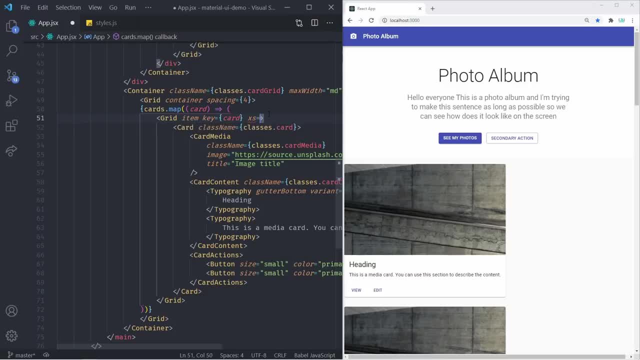 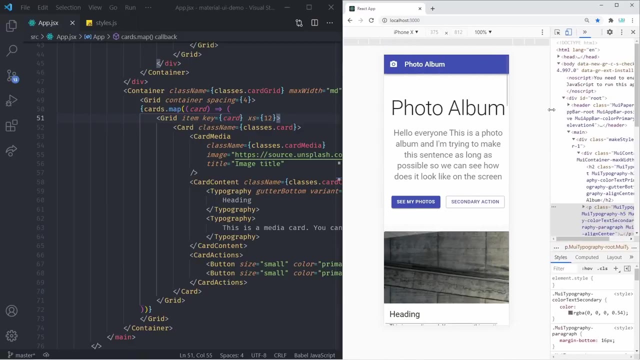 on a specific device size, So we start by extra small. These are mobile devices. On mobile devices, we want to take the full width, and the full width is 12 spaces. So you can see now it's taking 12 spaces And if we go to the mobile view, this is exactly what you want on mobile. 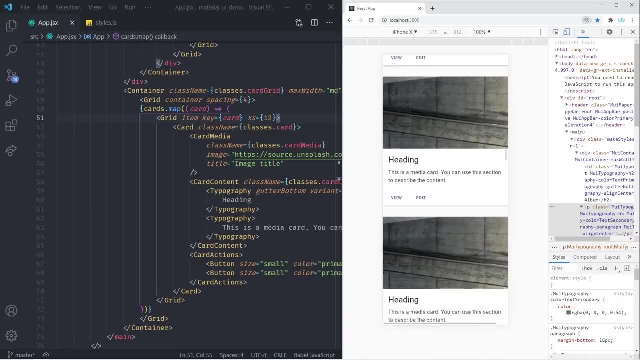 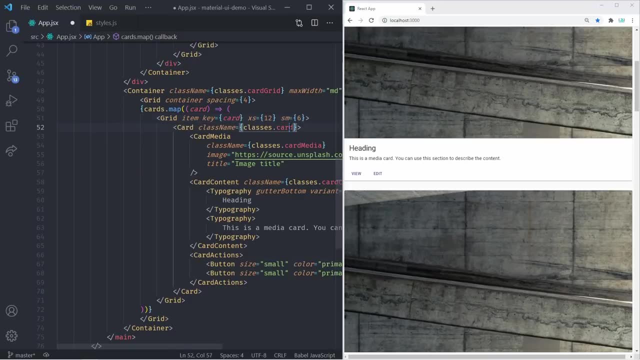 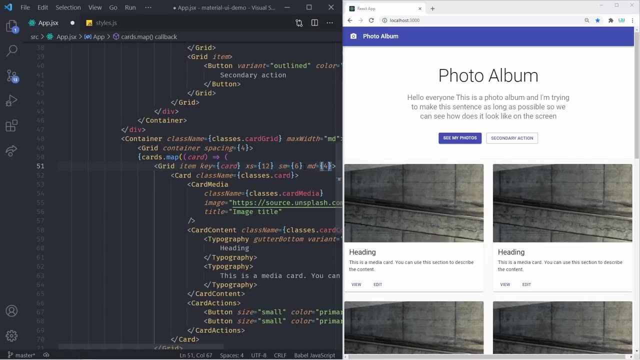 You want it to take the full entire space because there's not a lot of horizontal space, Okay, But if we are on small devices and larger, we want it to take half, because there is a lot of horizontal space. On bigger devices than medium, we want to use four, because 12 divided by four is three. 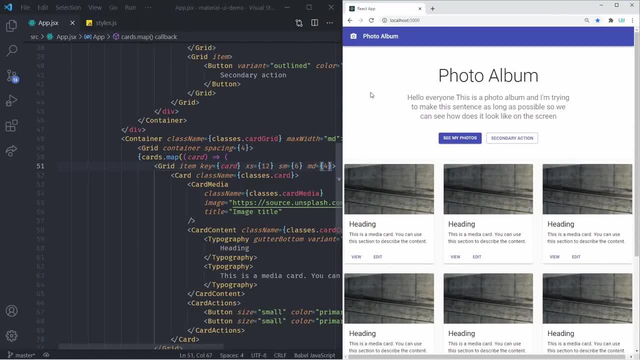 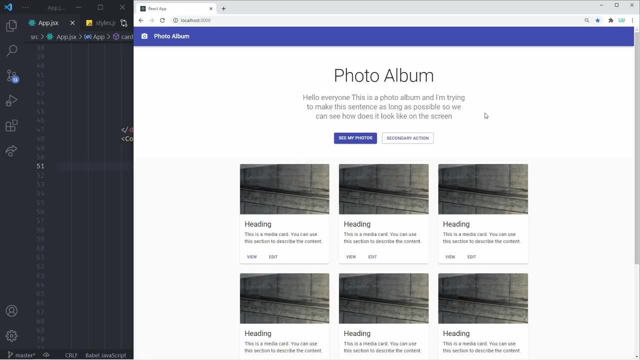 That means that we'll show three cards per row And just by this you immediately have a responsive design. You can see how it scales. We have three images on bigger devices And as soon as we start moving We get from mobile, we have just one. 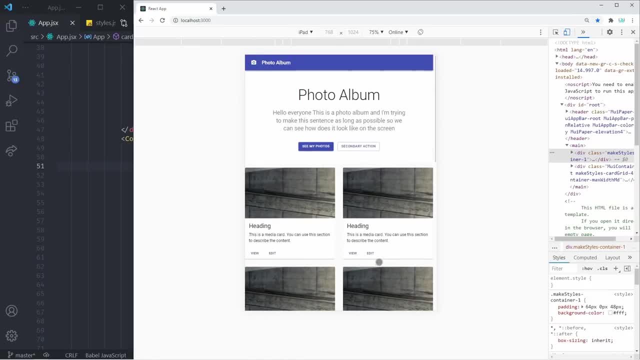 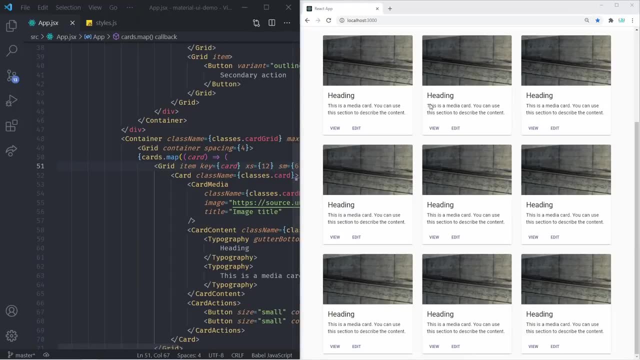 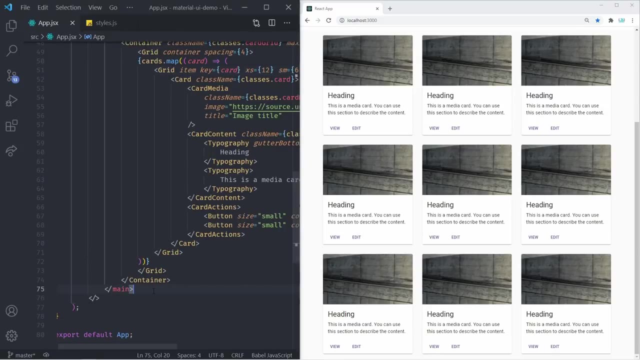 And if we go to something like an iPad, we have two per row. This page is fully and 100% responsive. The last thing that we need in this page to make it look complete is going to be a simple footer. So just below our main, we can create a new HTML5 semantic tag, which is footer. 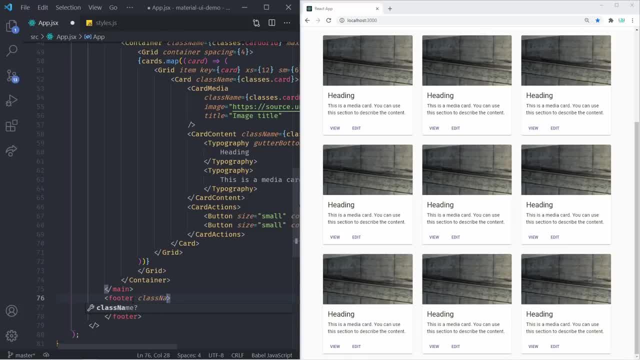 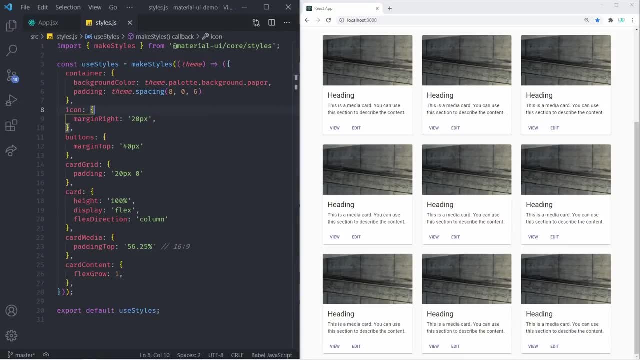 Inside of there, we'll give it a class, which is going to be a class name equal to classesfooter. While we're here, we can also just simply add that class, And it's going to be nothing more than a simple background color. 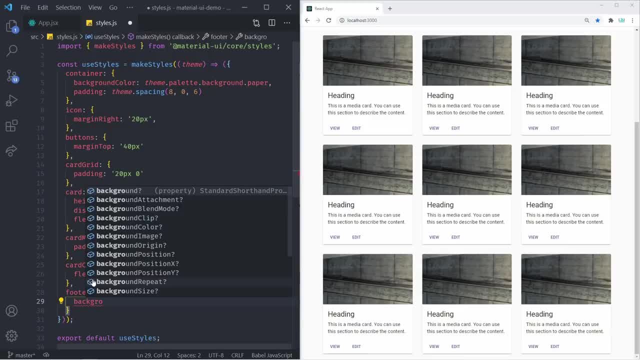 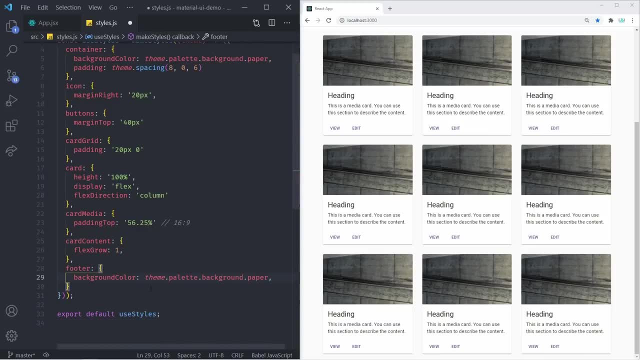 So we can go ahead and say: footer, give it a background color, And that background color is going to be the same as this one, So it's simply going to be a whitish color. And then we can also give it some padding, so we can see padding is equal to. and let's 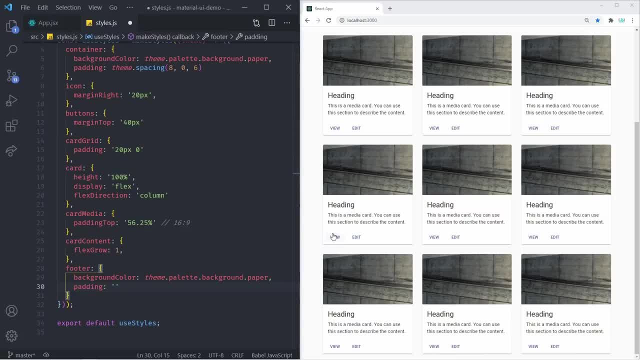 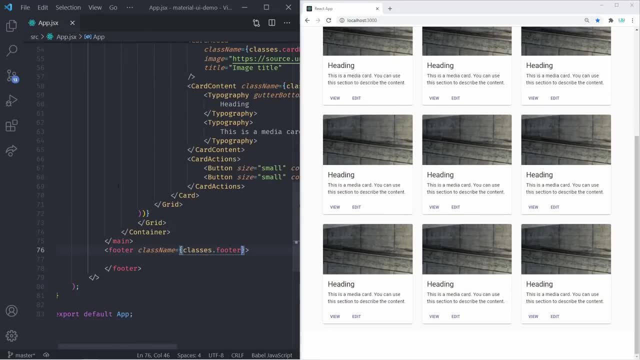 do something like 50 pixels on top and bottom, So we can say 50 pixels and then zero on left and right. Okay, with that said, we can start implementing that padding And that's going to be really straightforward. It is going to have a few typographies. 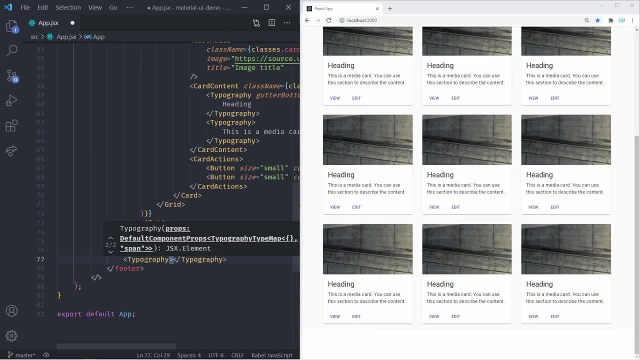 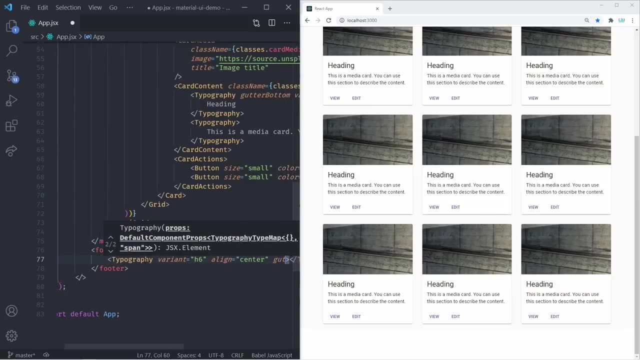 You can already see how typography is a really useful tool that you can use in Material UI. We're going to give it a variant of something like let's do H6.. We're also going to give it an align of center And we are also going to give it a gutter bottom. 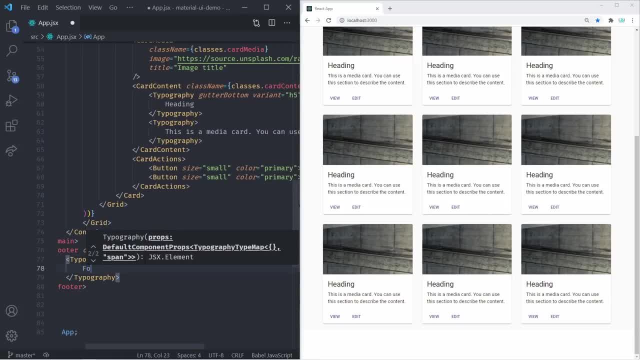 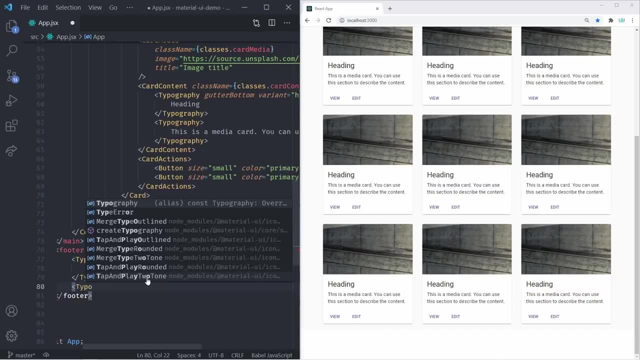 Okay, finally, this is going to say something like footer. That makes sense. Okay, and we're going to have one more typography below this one. This one is going to have a few different properties. We're going to use a variant which is equal to subtitle one. 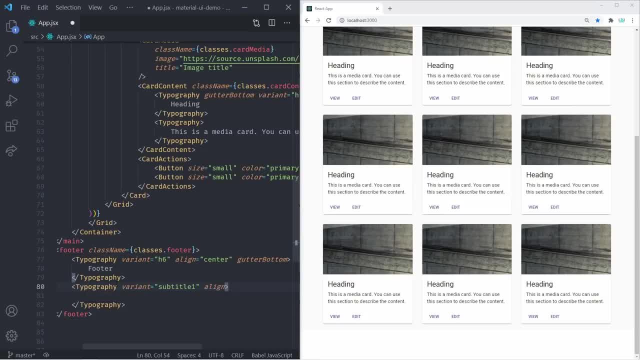 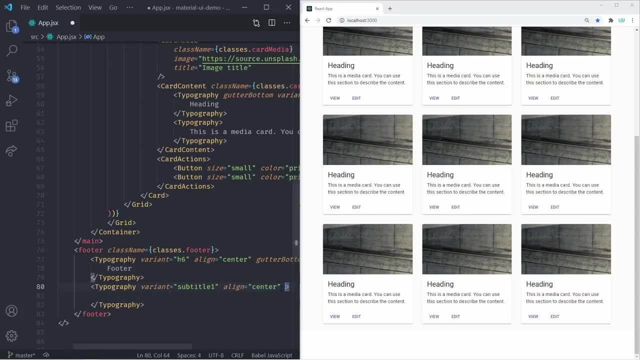 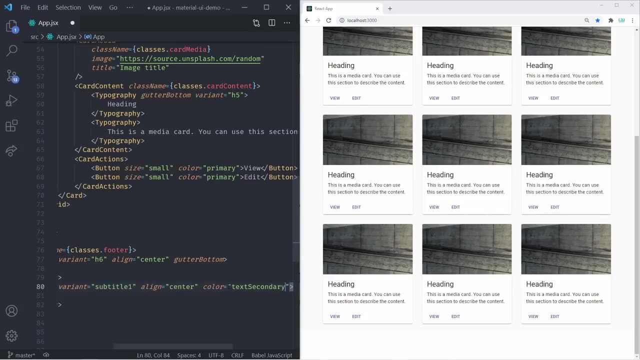 It is going to be aligned to center as well, So align center. It is going to have a color of text secondary. It's not going to be so prominent, So we can do. color is equal to text secondary And that's going to be it.